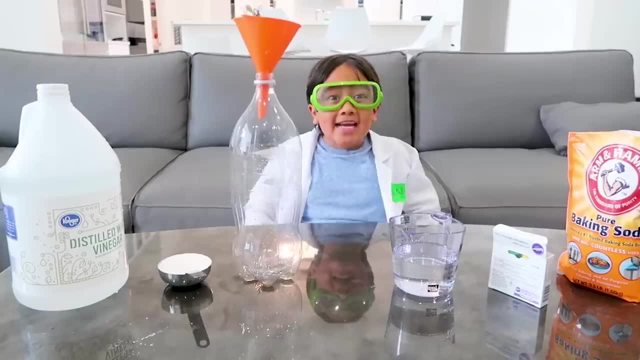 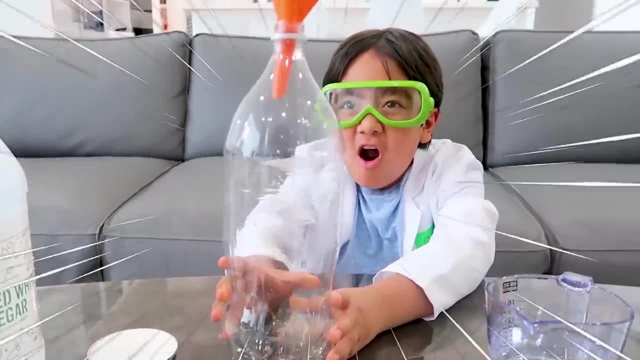 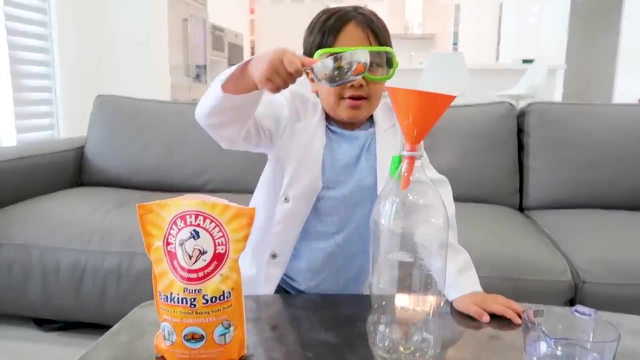 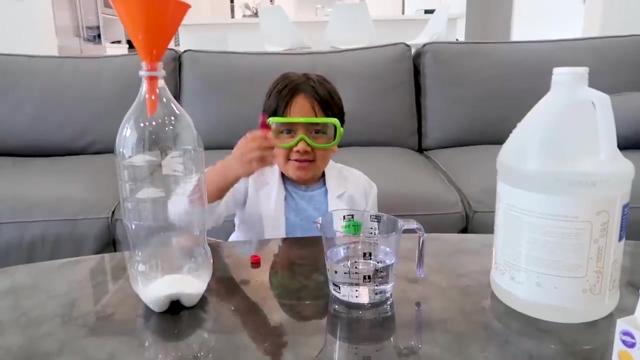 Hey guys, today we're doing the baking soda and vinegar science experiment. But first pretend this is a volcano. First you're going to need some baking soda, So we have to put it into the funnel inside your water bottle, Okay. next you're going to put your food coloring into your vinegar, and I choose red. 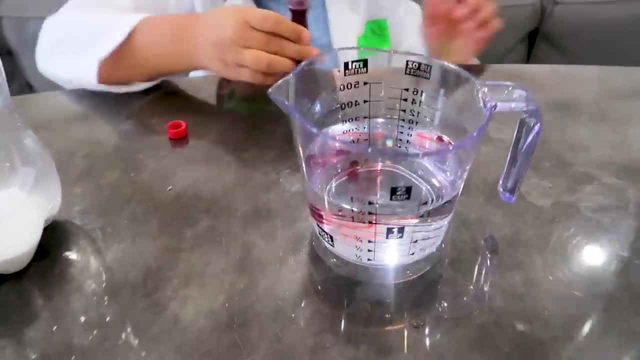 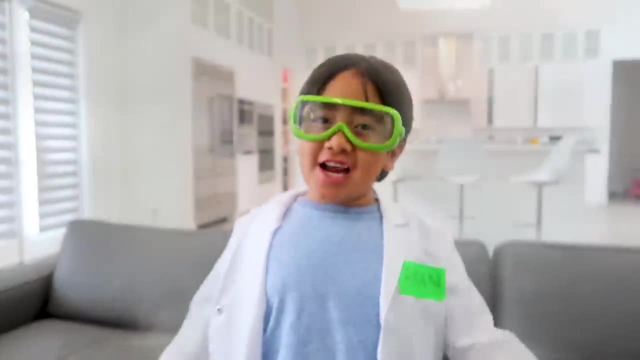 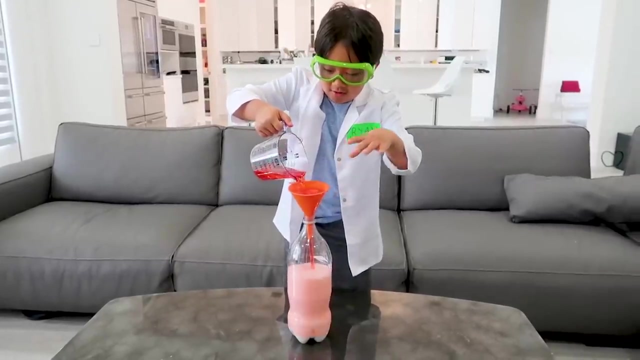 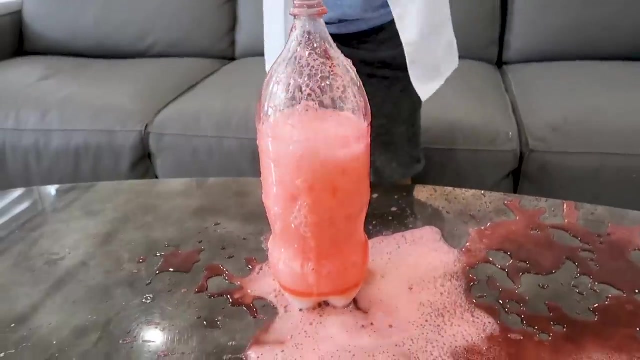 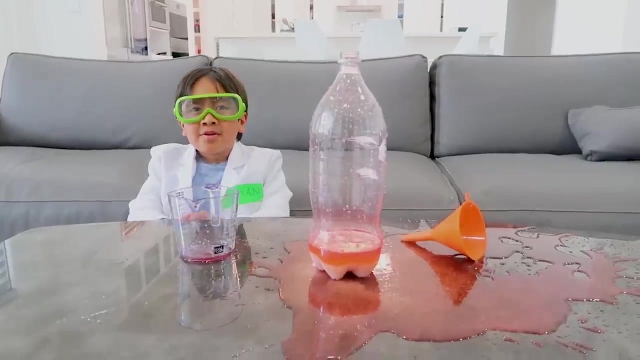 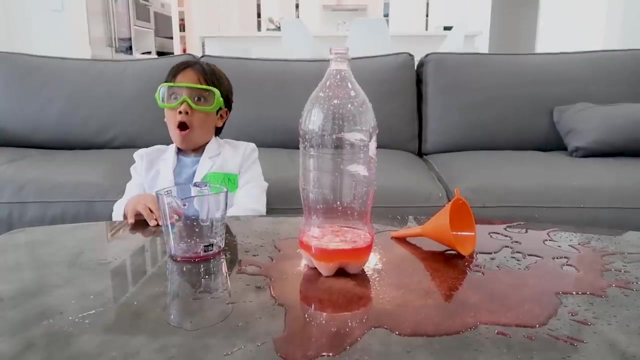 A little bit more. Okay, guys, get ready for an experiment. Remember, ask your parents for help. Whoa, that came out. That was so cool. That was really fun, but I wish it was a volcano. Huh, Peck, Hi, Peck. 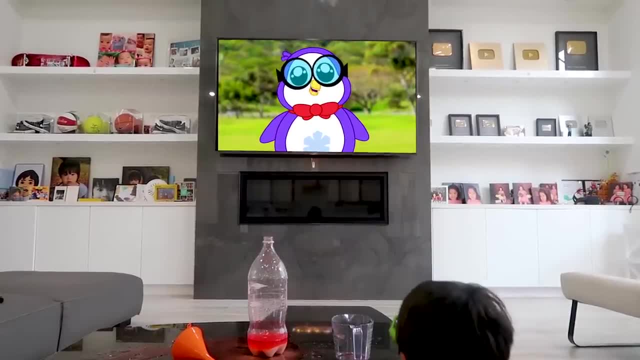 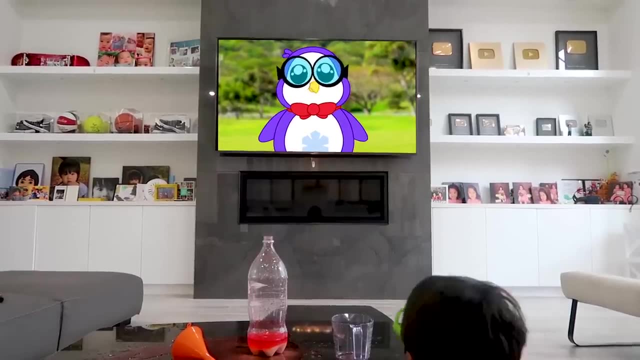 Gosh Ryan, did you know that you can make a volcano out of paper? What You can? Of course you can. I'll go make one for you. Okay, I'm going to build a Lego robot. It's going to be my best friend. 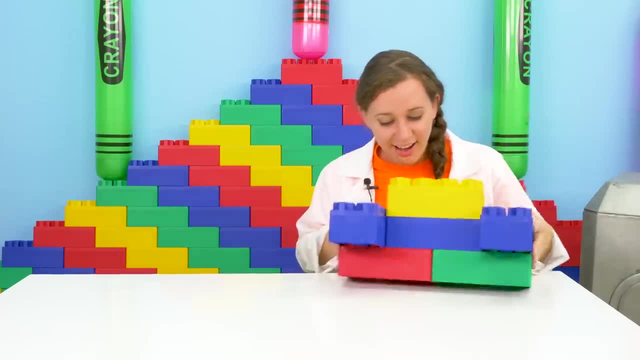 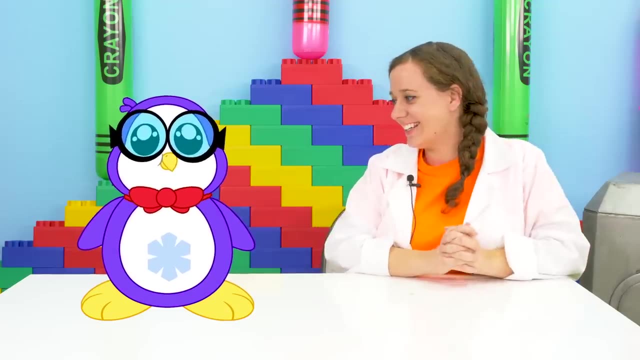 All I need is the last piece, The last piece for the head, and Oh, it's so cute. Whoa, whoa, whoa Peck. what are you doing here? We got a new science experiment for Ryan. It's going to be a giant volcano. 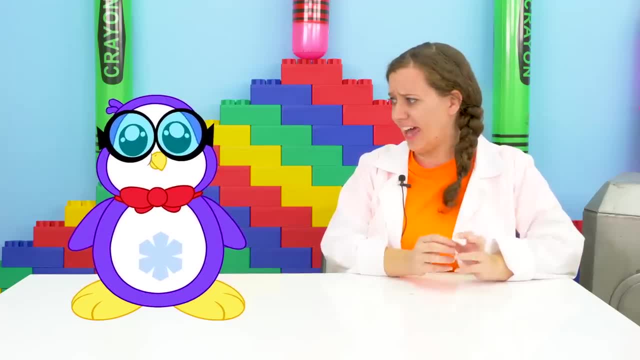 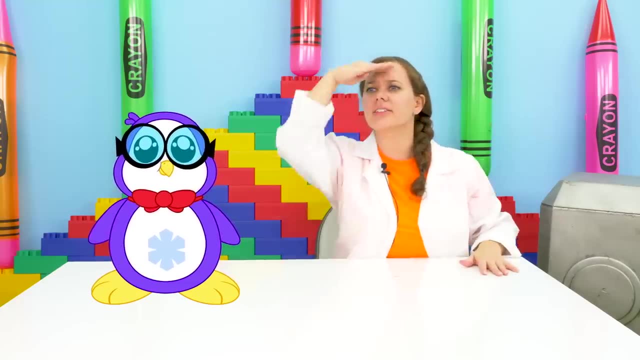 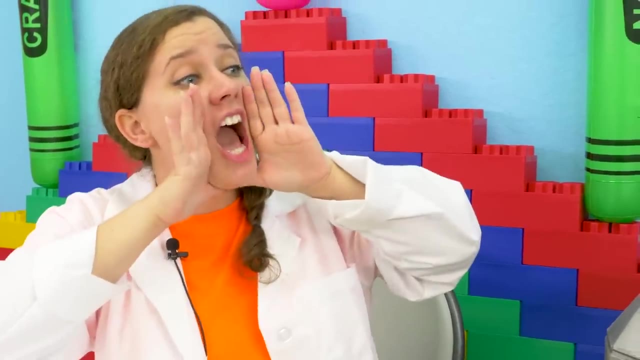 A giant volcano. Well, what do we need for that? First thing we will need is a giant box. A giant box. There's definitely one around here, Let's see. Oh, over there by Combo. Hey, Combo, pass the big box. 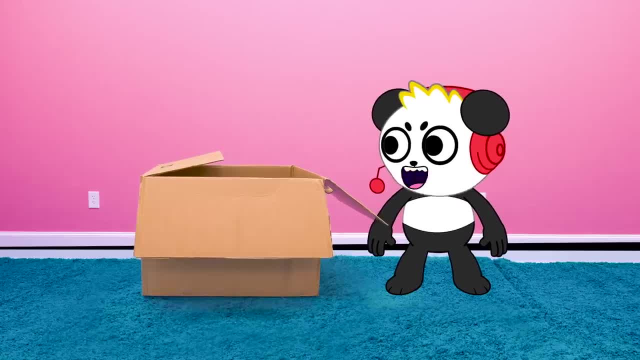 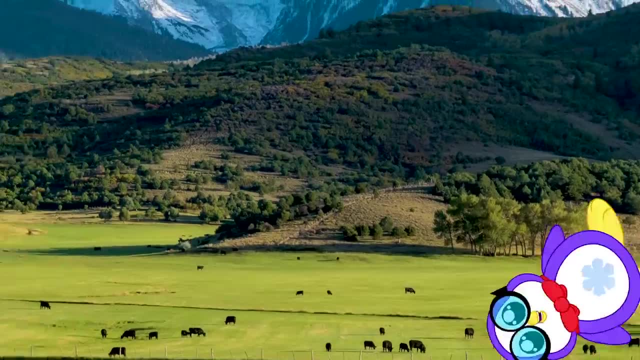 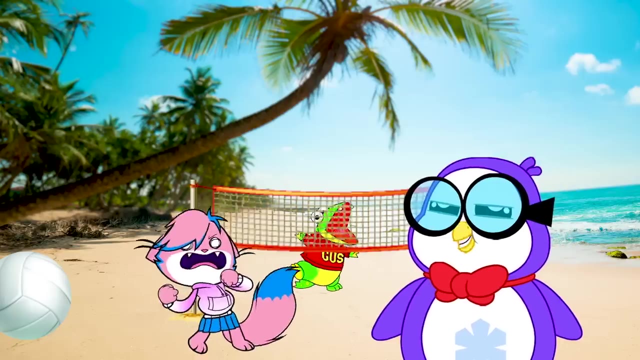 Huh, Oh, this box. You got it Bree. I'm a little teacup shark. Whoa Yeah, Whoa Yeah. perfect. This place doesn't seem too familiar. Huh, What's that? 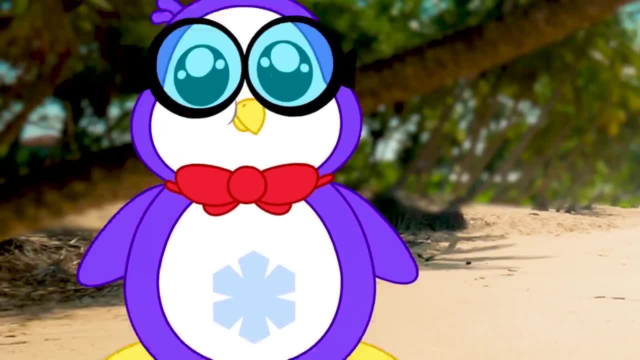 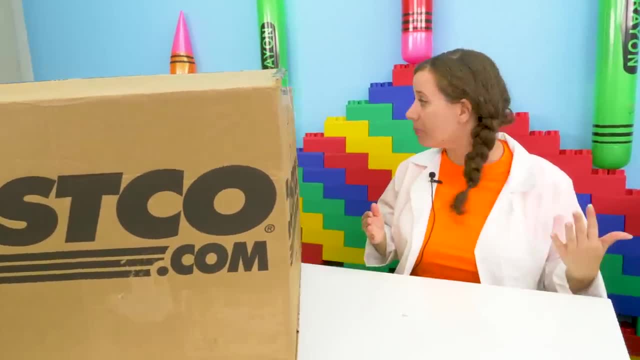 It looks like there's a volcano nearby. Let's go investigate. Whoa, This box is huge And it is going to be the perfect base for our volcano, Don't you think? Peck, Peck, Where did Peck go? 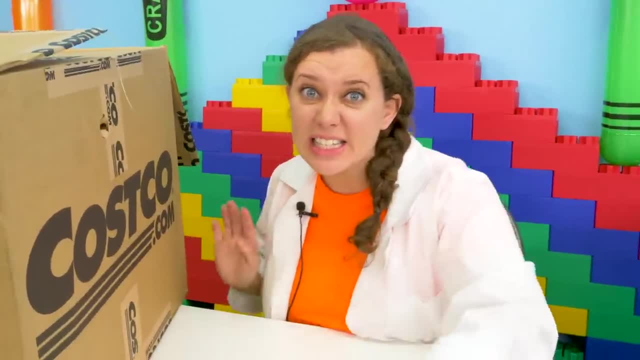 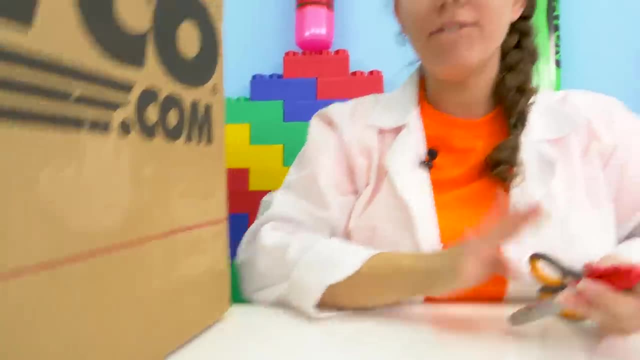 Oh well, let's get started. The first thing we need to do is cut this box down, So I finished marking my line Where we need to cut. it's about four inches high, which I think is going to be a good height to keep all the lava inside. 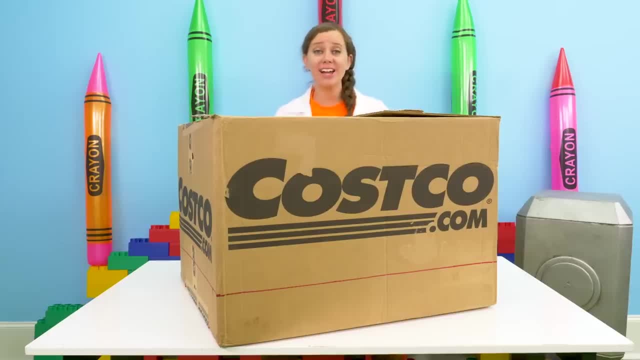 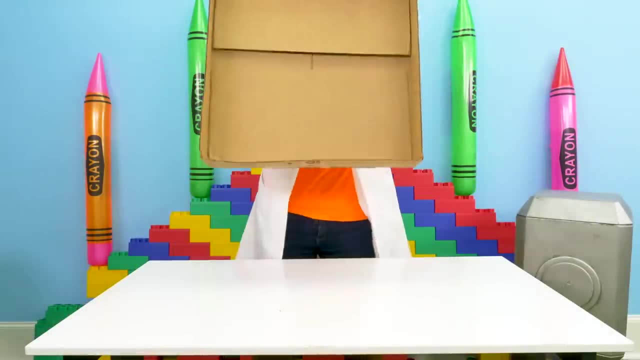 So now all we need to do is cut, And once we cut the box, it should look like- And there it is. That is the perfect size for our base. Look how big it is Now to make sure that our base is good and strong. 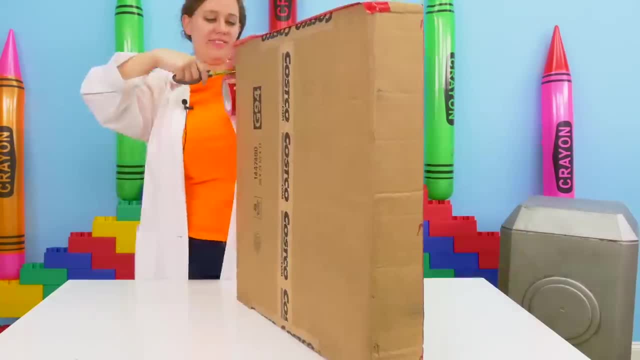 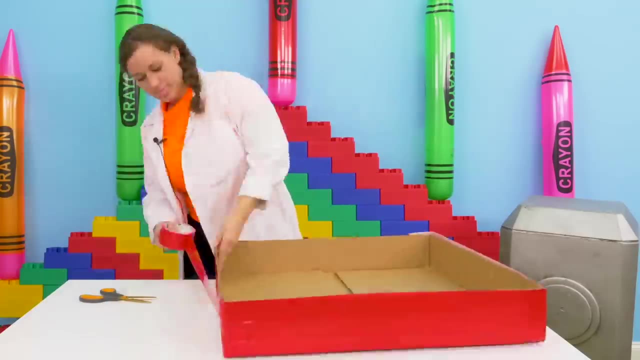 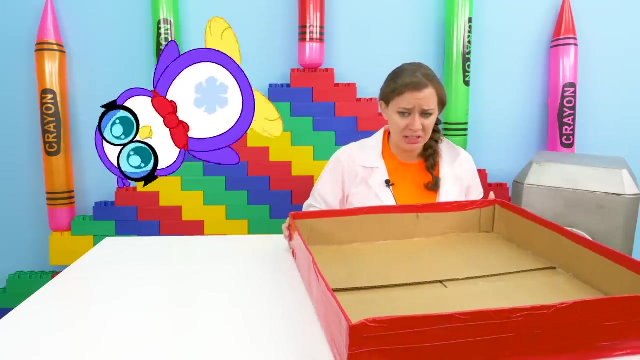 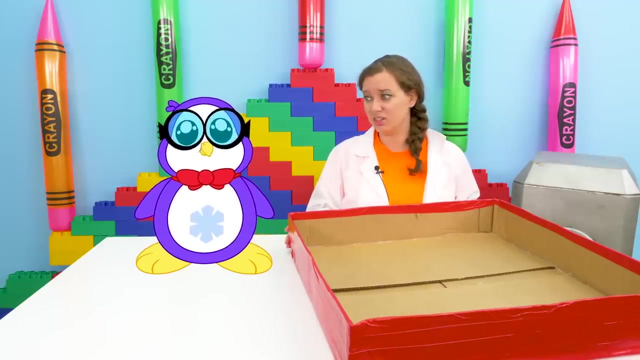 we're going to use duct tape. Well, the box looks great, but how do I build a volcano Incoming? Oh Peck, there you are. Huh, I just got back from gathering research data. First, we're going to need these. 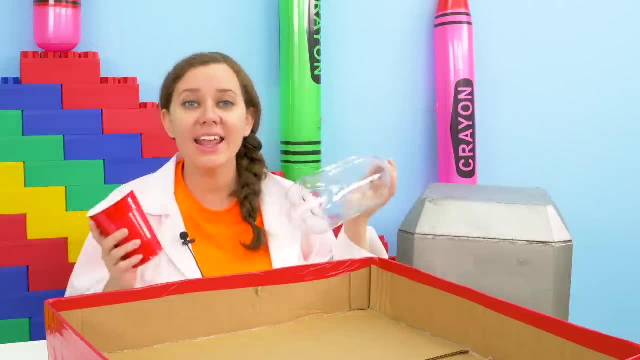 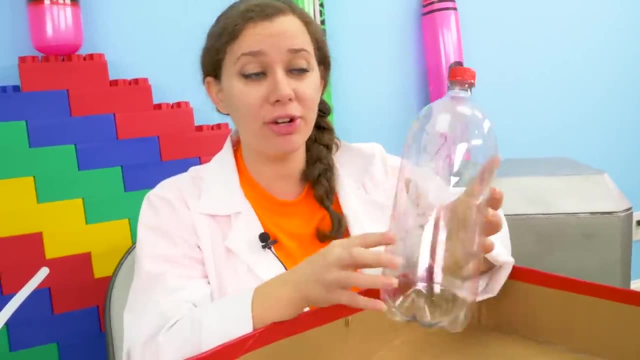 A bottle and a cup. I think we can use this for the center of our volcano, Precisely So. this bottle is going to be perfect to put all of our ingredients in for the lava, But I think it's a little too big. 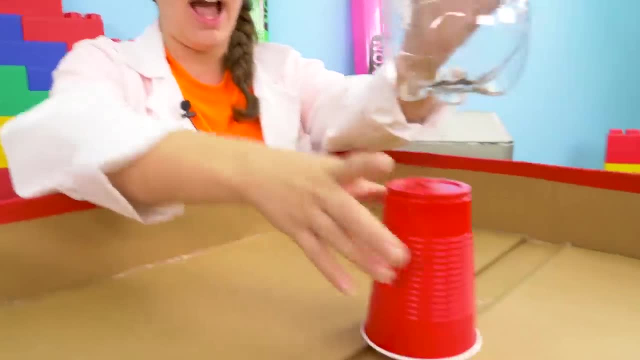 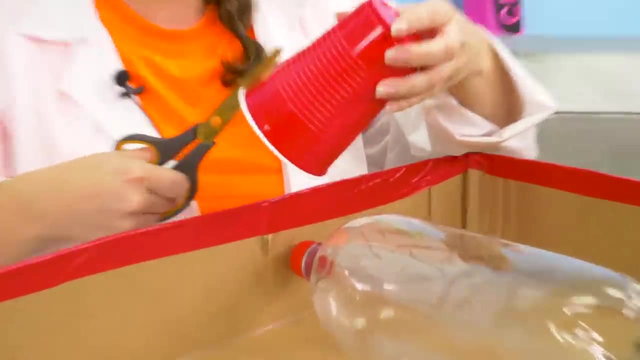 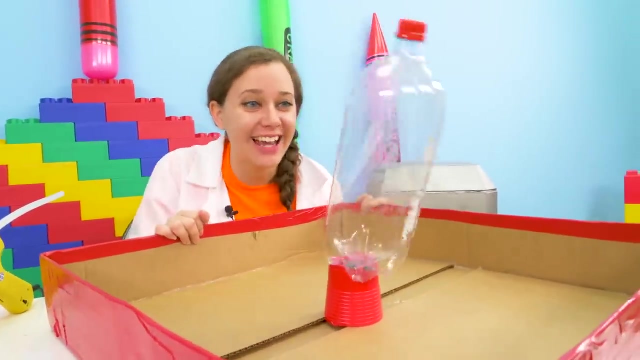 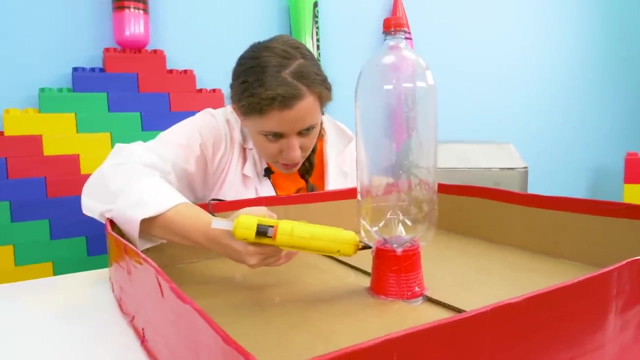 I think it's a little too short. That's why we have this cup. I think that might be a little too tall. We can work on this. That is the perfect height. Maybe we should glue it in place. Okay, just a little bit more glue. 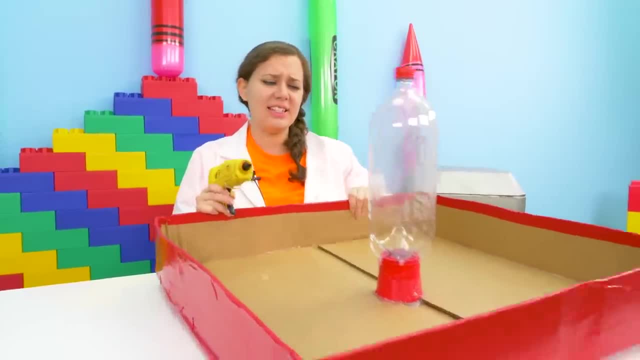 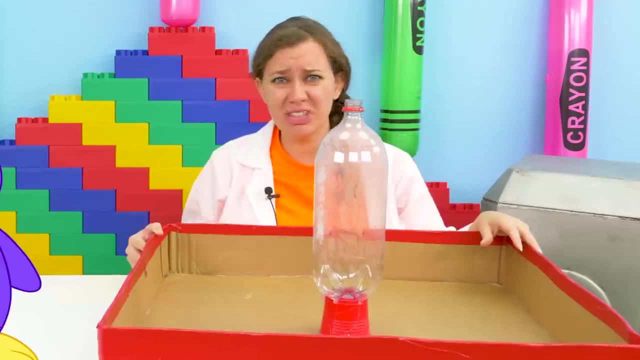 And I think that should do it. I don't think it's going anywhere. Okay, our bottle's not going anywhere, but we don't need this cap. It doesn't really look like a volcano. We need something, I don't know what. 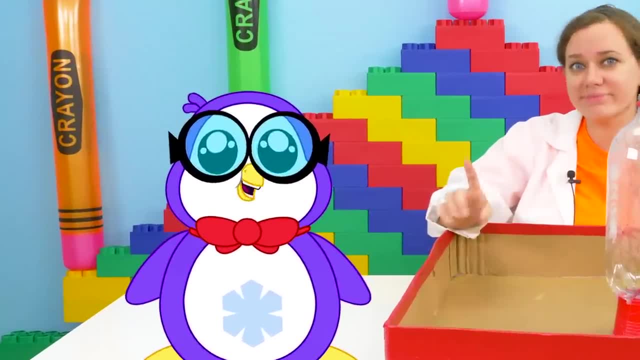 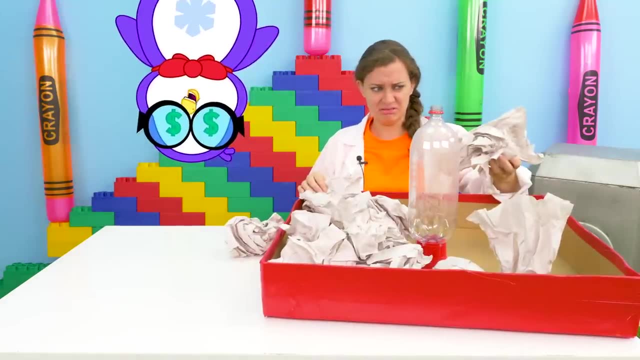 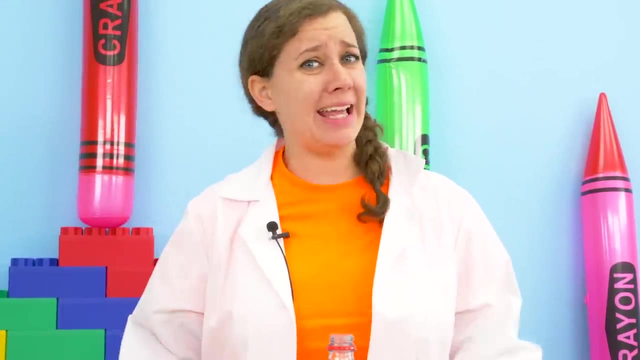 We have to build a body. I know what'll work. Okay, Nyah, Trash Paper- Oh, that's a great idea. So we're making the shape of our volcano. It's kind of a mess though. It's kind of a mess right now. 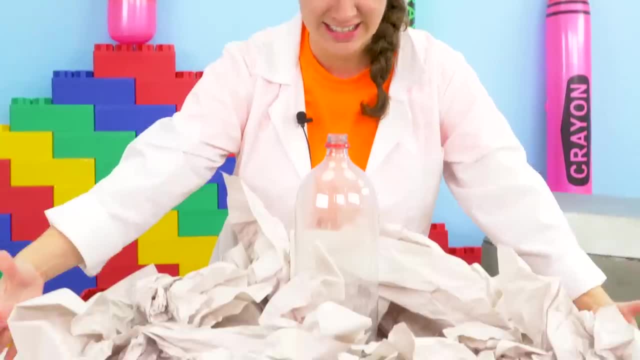 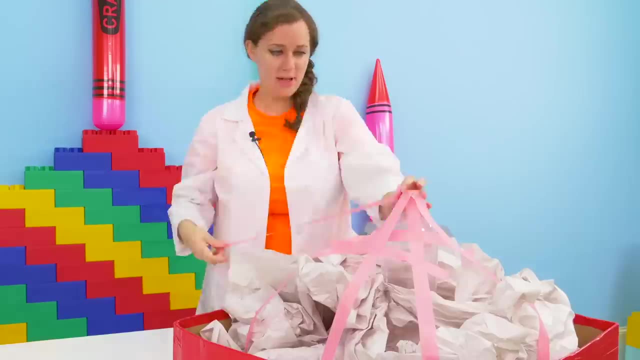 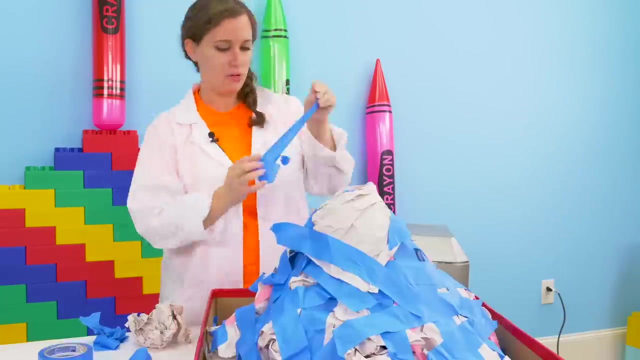 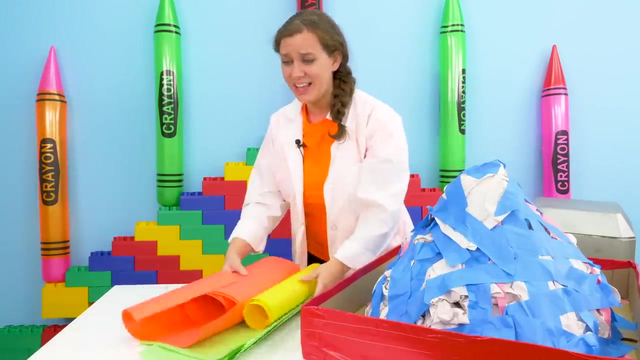 So we're going to use tape to hold all of this together. Now to form the body of the volcano. with some tape, More paper, Whoa Wow, Peck, you found a lot of paper. This is going to be perfect. 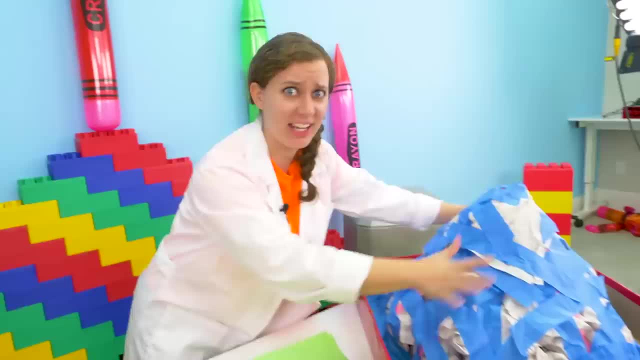 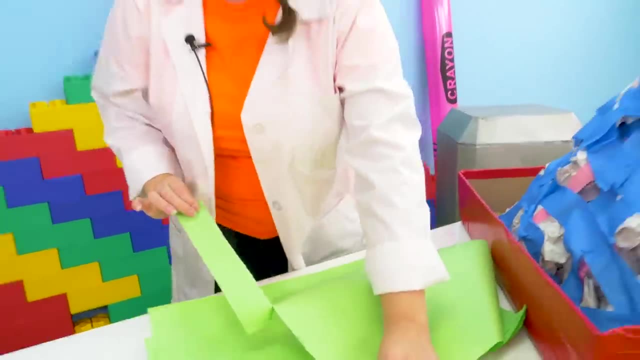 So the first thing that we need to do to start paper machining- this giant volcano- is we need to take all of this paper and tear it into pieces that we can actually use, So something about like that. But we're going to need a lot. 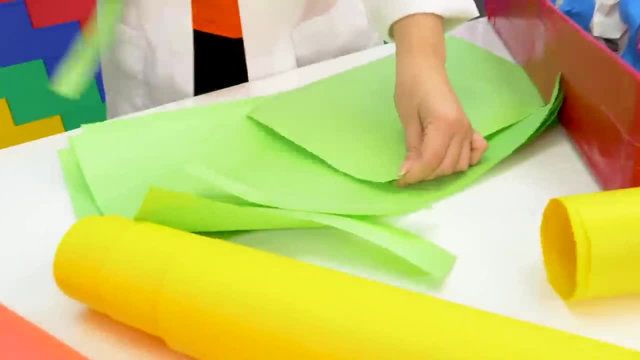 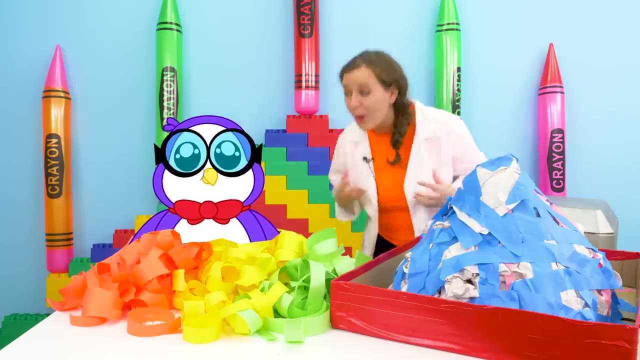 This guy is very big, so, Yeah, This ought to do the trick. Rip the paper, Whoa Peck. great job, This is a lot of paper. What else do we need? Uh well, to make it, we're going to need: 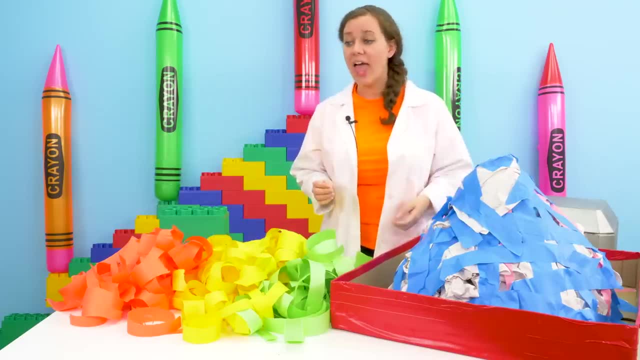 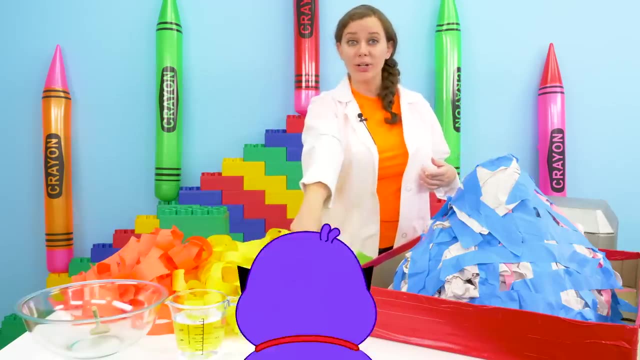 Well, to make paper mache, we need paper, which we already have, and then we need a bowl, some water and, the most important part, glue. So this glue is way too thick. So the first thing we're going to do is add glue. 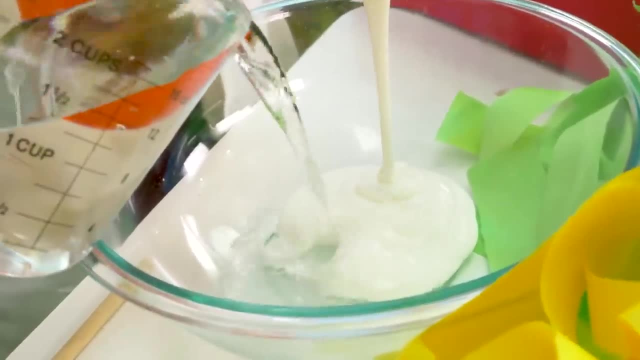 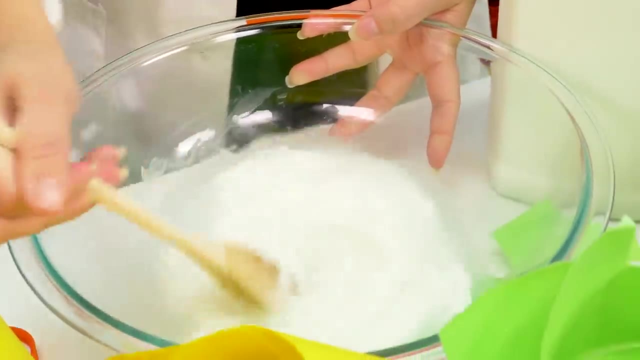 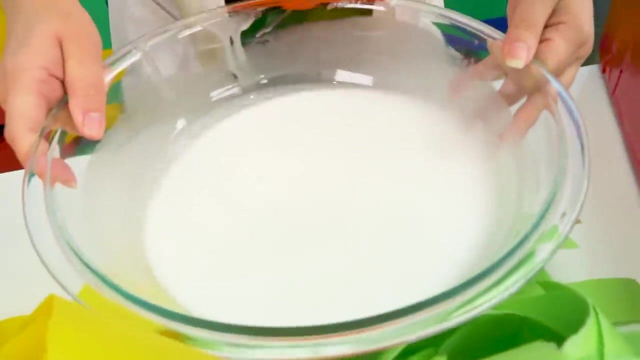 Then we're going to add water and stir it all together to try to thin it out so we can put it on our paper. Now all we do is stir Or agitate, Agitate, Agitate, And when you're done, it should look something like this: 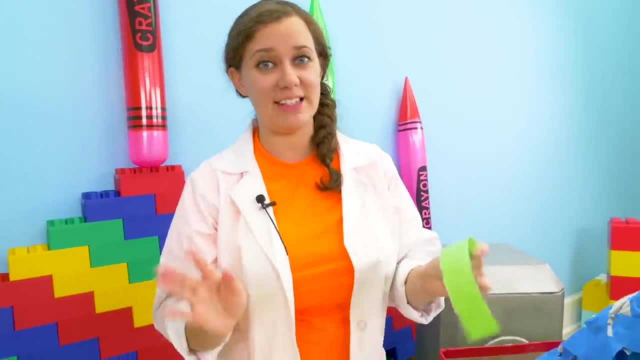 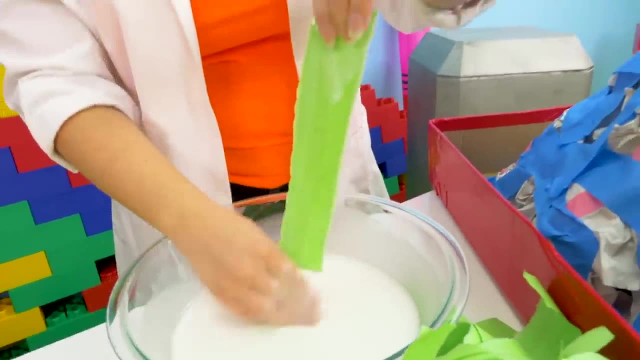 Now we're all ready for the fun part. It's going to be a little messy, so if you're wearing sleeves, roll them up. First you dunk it in the glue And then you just clean off all the extra. Make sure the paper is good and kind of soft. 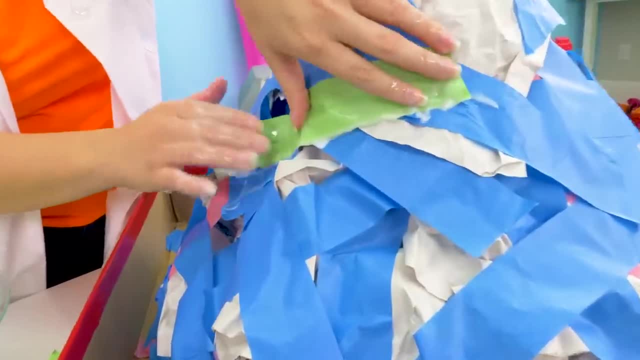 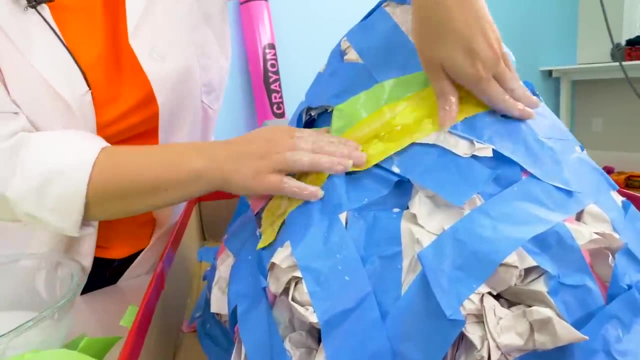 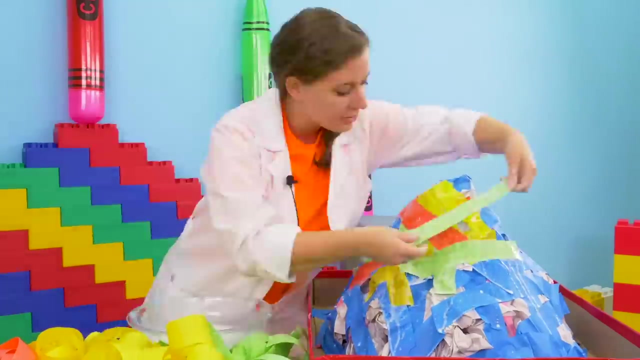 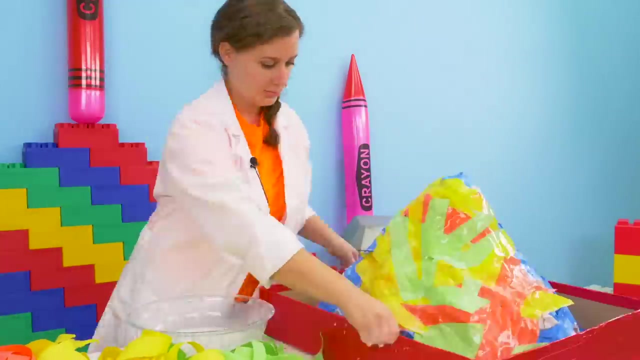 And then you just slap it on the volcano And then anymore you're open, So you can just let it dry for a couple minutes And then you can just remove the paper. It's as easy as that- Slimey Slimey. 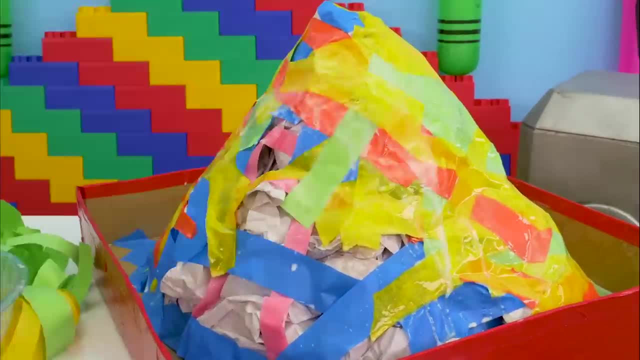 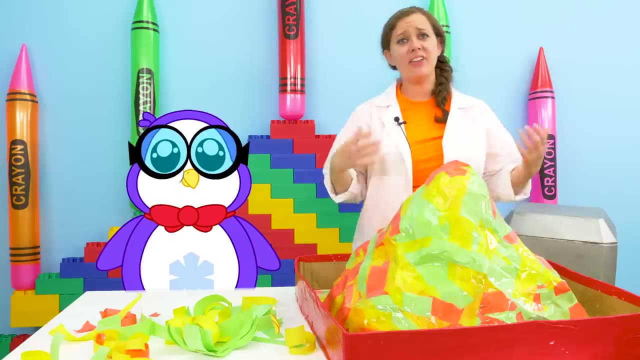 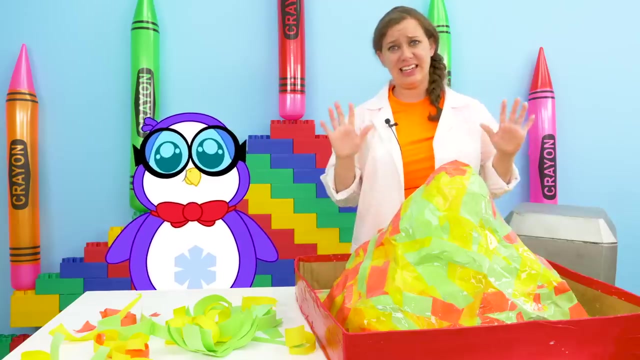 Slimey, Slimey. Now the hardest part: we have to wait for this to dry. It's going to be hard at first to dry. the volcano will take a while to dry. let's go wash our hands. uh yeah, i'm very sticky, so we'll. 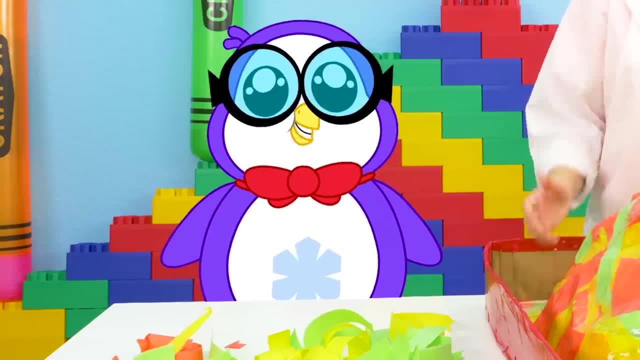 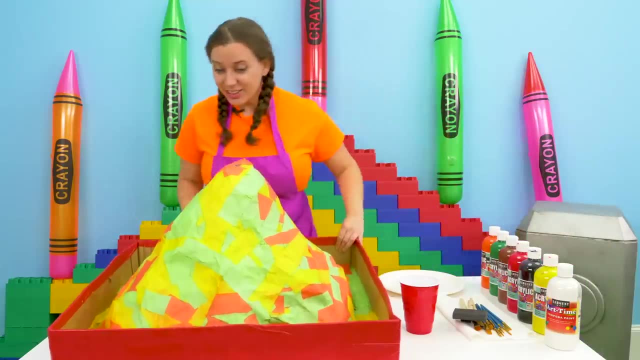 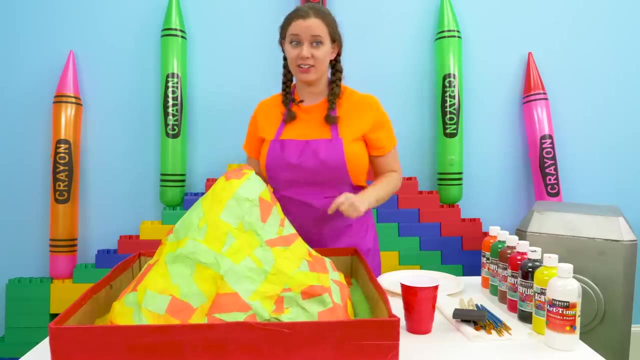 meet back here later. yup, i'm gonna go gather more research. bye one day later. whoa, it looks so good and it's really dry. let's see. it's definitely hard and sturdy, ready for paint, but where is peck? peck, are you free peck? oh yeah, i'm at a real volcano and um. 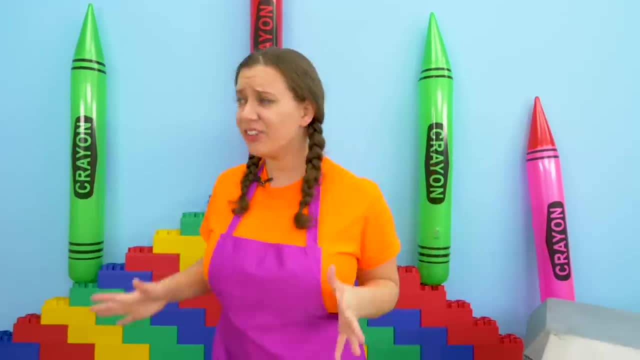 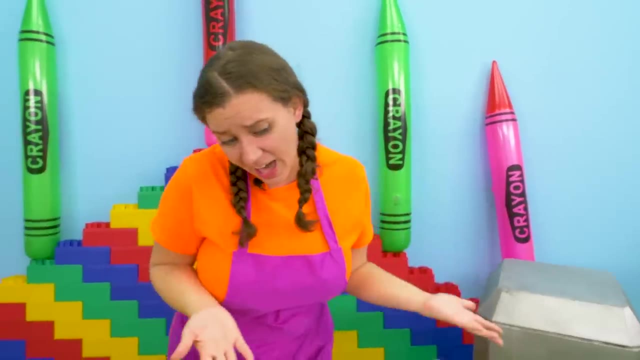 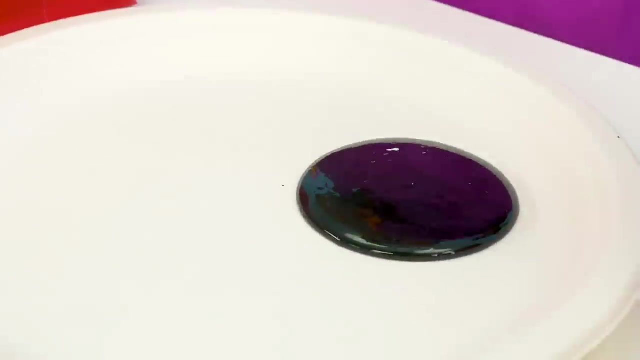 i think we need to use a gray paint. well, we can definitely make gray peck, but just make sure you stay safe. okay, be careful. now, gray we don't actually have, but we can make it with black and white. all right, peck. uh, how do these grays look? 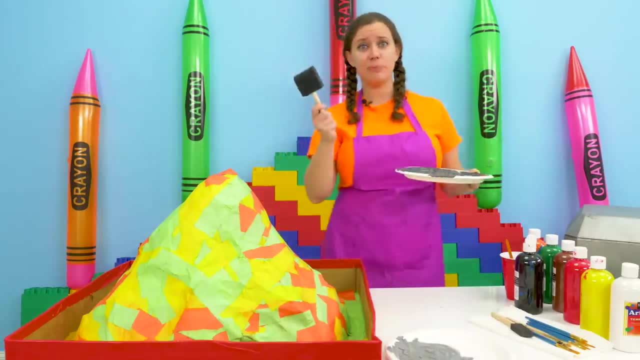 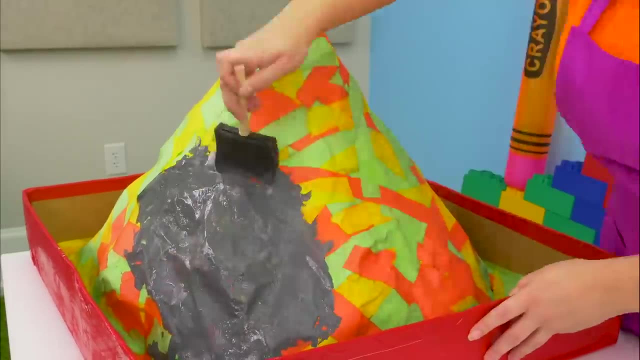 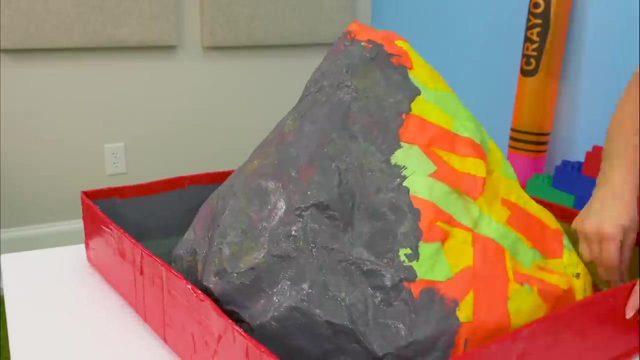 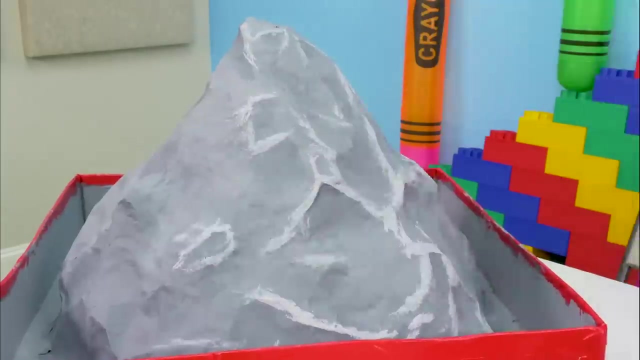 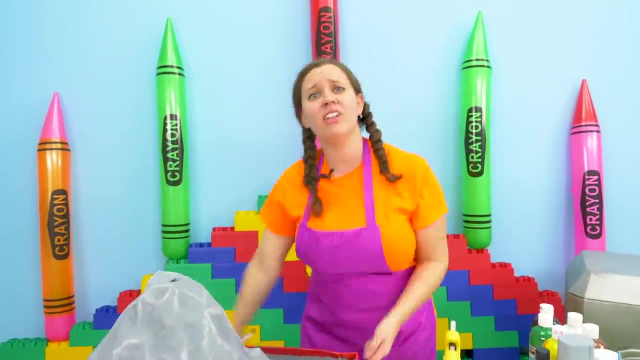 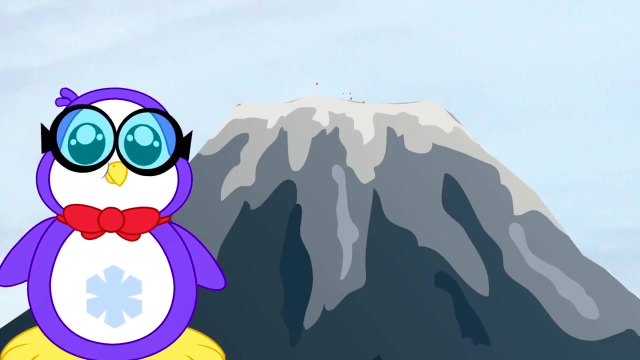 all right. well, it's a big volcano, we're gonna use a big brush and let's get started. all right, we just finished all of this painting. this volcano is huge. it took forever peck. how does it look? it kind of looks just like a mountain. it could use some lava, some lava. oh yeah, awesome lava. i'm gonna. 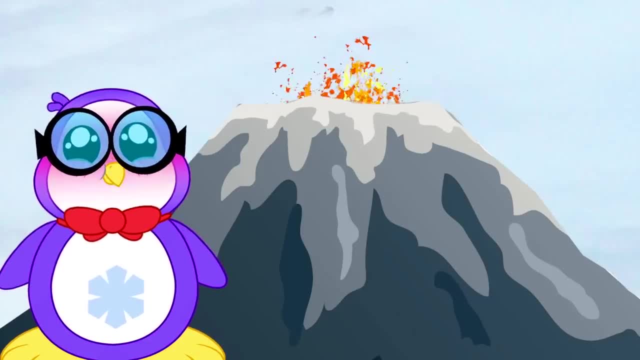 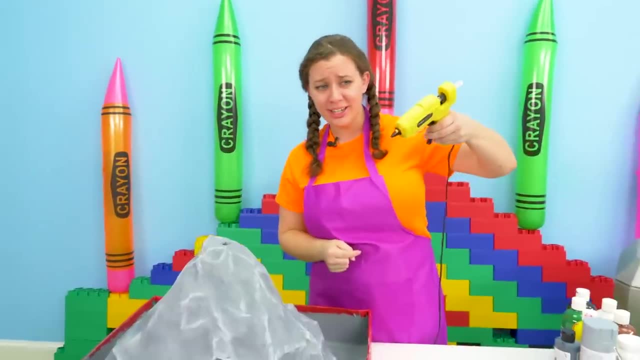 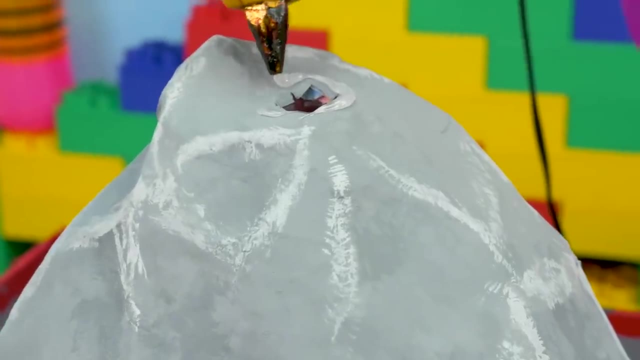 head back. now. it's getting a little hot over here, okay. well, we'll see in a bit peck now. i have a great idea for the lava. what better than hot glue? i mean it kind of looks like lava, right, maybe? all right, let's see. so we're gonna try to build it up and see if we can get it to look like some big. 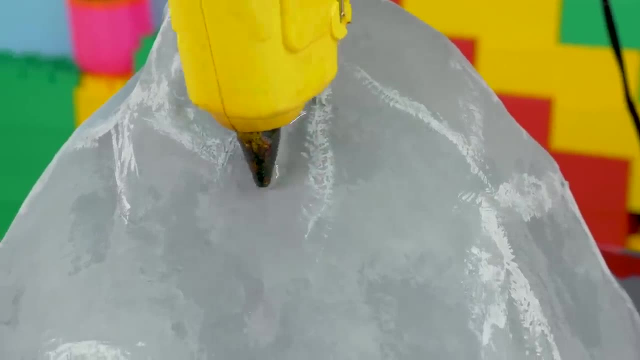 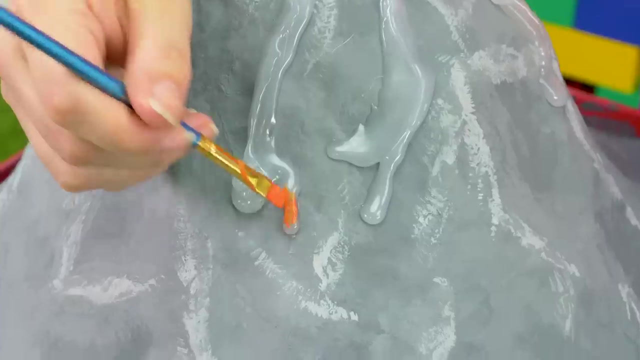 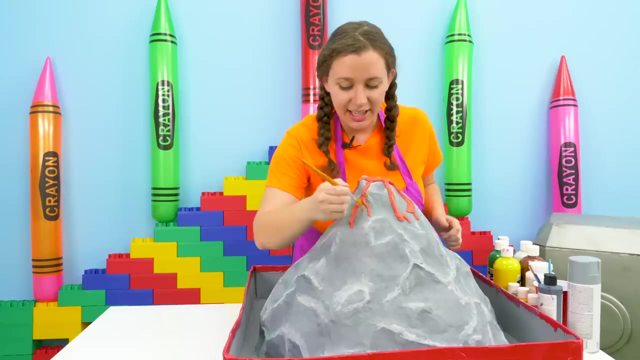 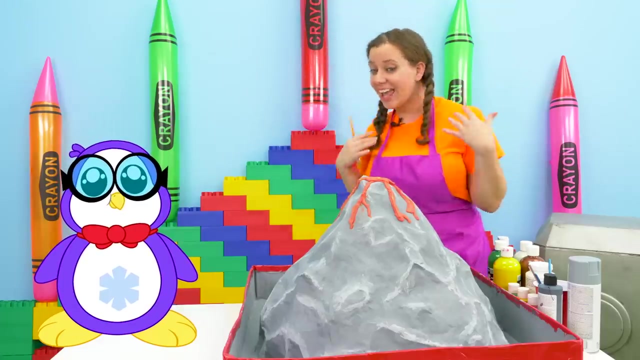 giant lava trails. whoa, that looks so cool. all right, now we're gonna use some orange and some yellow to give this lava some color. oh, just a little bit more lava paint, and i think i hear peck made it just in time. oh, hi, peck, so we just finished our volcano. and what do you think about? 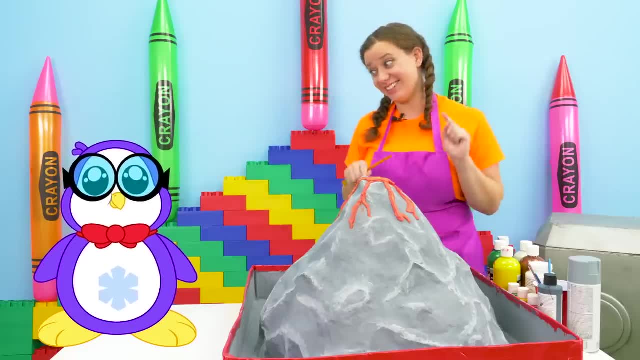 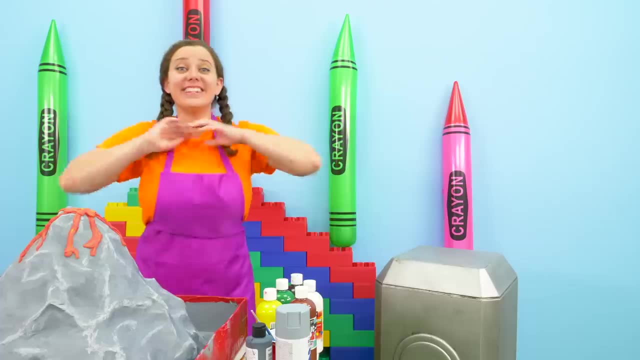 it. i think our volcano is complete. looks like the real deal. huh, looks like the one i saw earlier. let's teleport it to ryan. yay, the last thing we have to do is to get this onto our teleporter- portator potato. so let's just lift this guy. 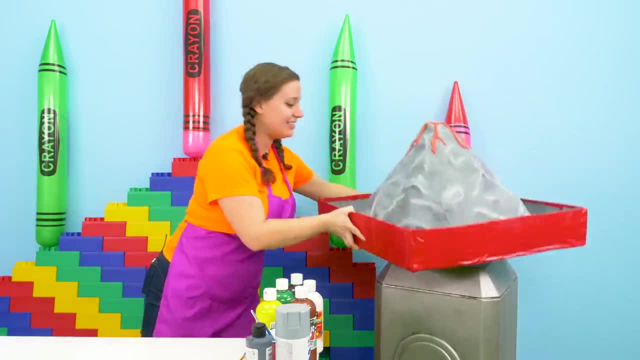 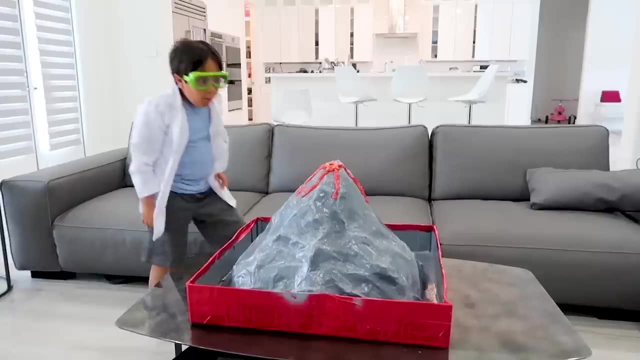 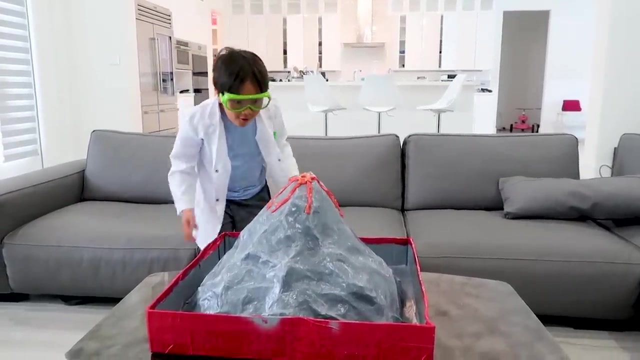 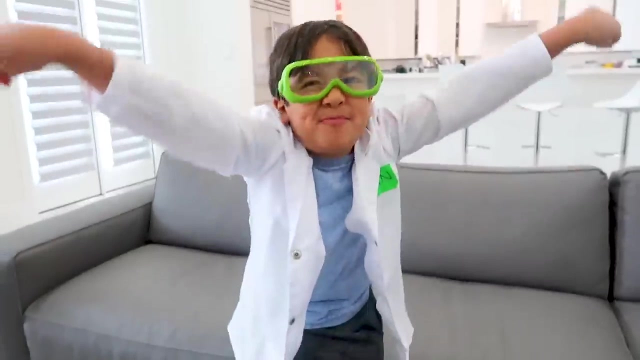 i'm just kidding, it's paper mache, it's really lightweight. and off to ryan we go. goodbye volcano, have fun, ryan. wow, thank you so much peck for this paper volcano. it's so cool, super cool. i'm gonna bring it outside and then i'm going to rock it. 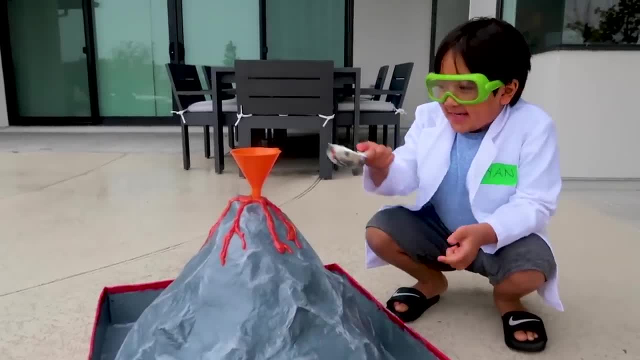 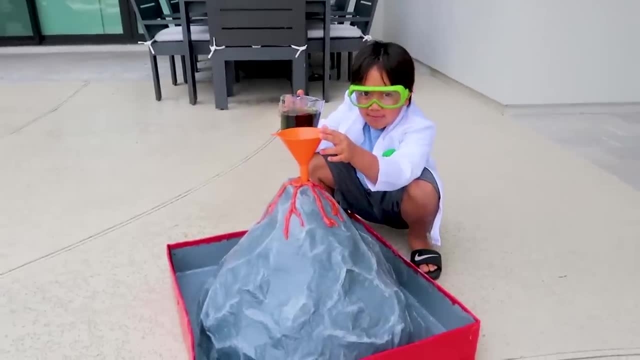 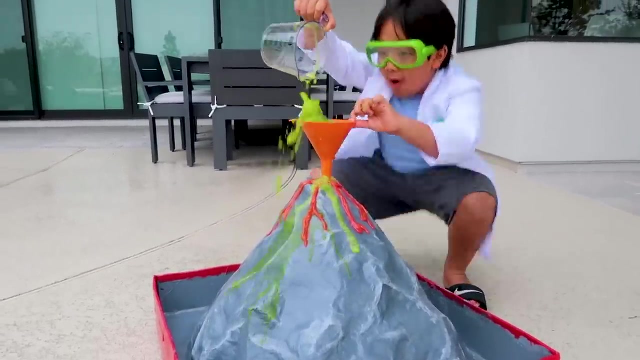 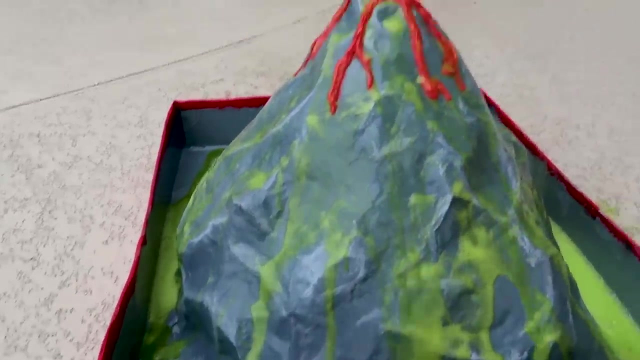 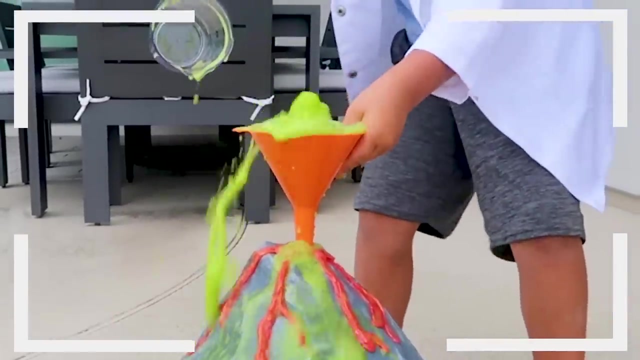 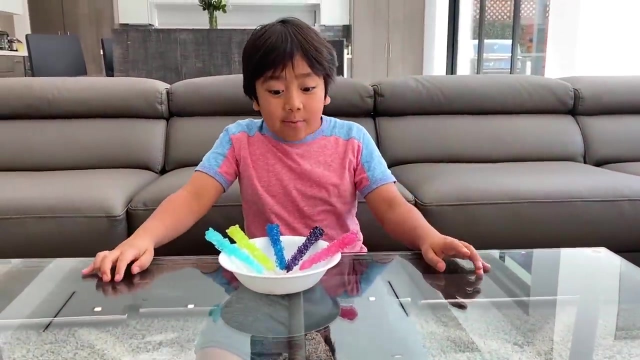 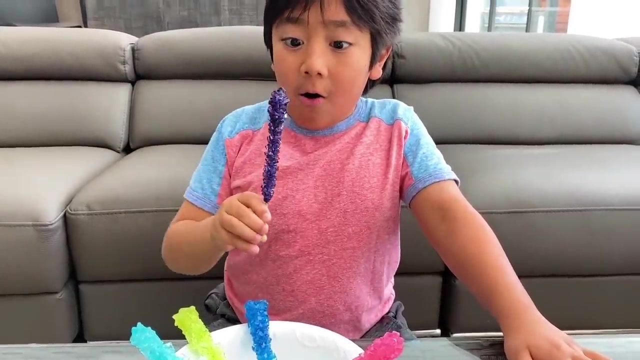 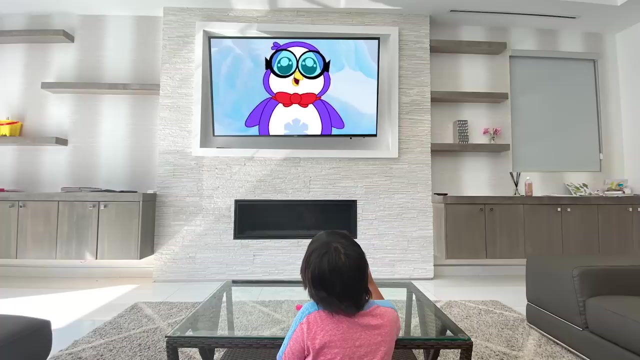 let's go. first thing, baking soda. okay, guys, so let's pour in the vinegar. whoa, whoa, there's so much green, green rock candies. i wonder where these came from. whoa, i wonder how these were made. hey, ryan, hi peck, did you know you can make rock candy at home. 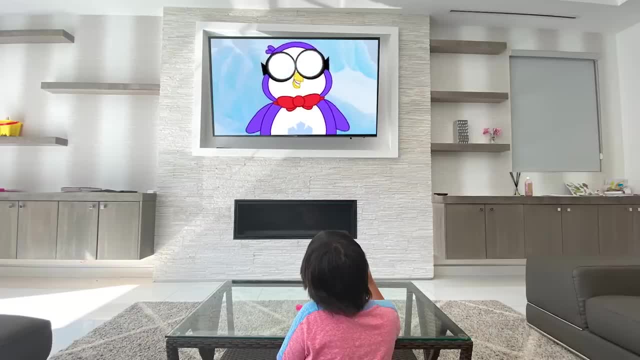 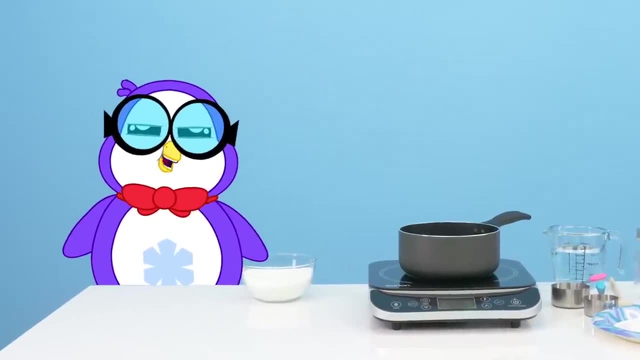 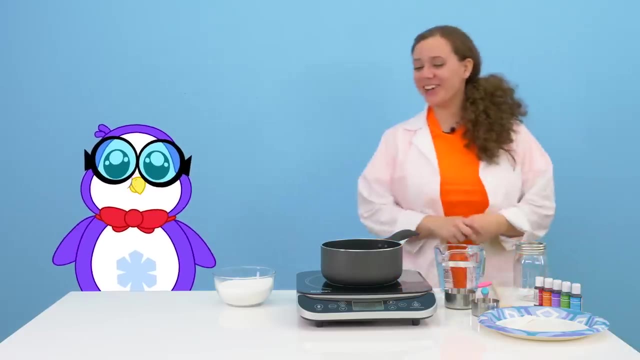 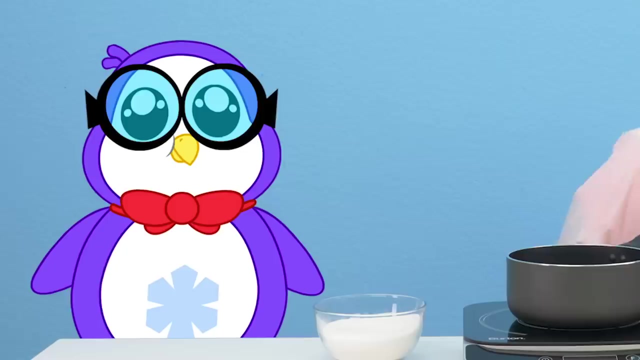 you can, yeah, you can, yeah, haha, you can, yeah, haha. want me to show you how sure, then let's go. okay, i got this, um, um, maybe just a pinch of sugar. hey, peck what you doing? oh gosh, definitely not eating sugar. uh-huh, this looks pretty cool what you got going on. 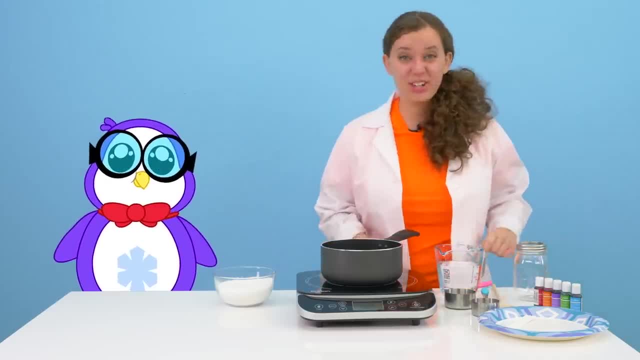 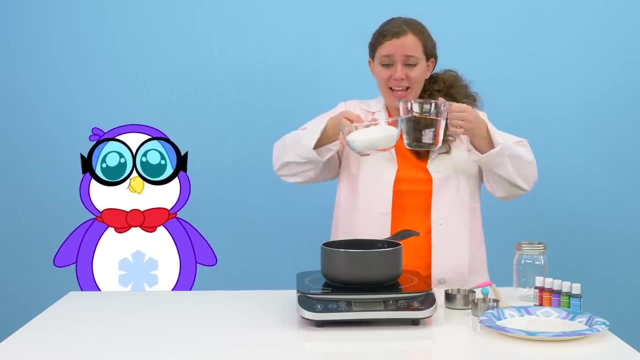 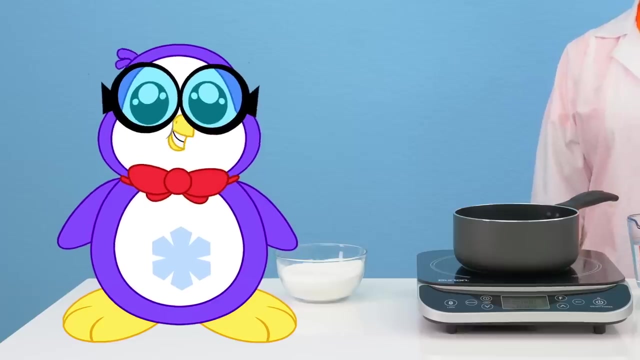 making some rock candy for ryan. oh, you know the best thing about rock candy: it's actually really easy to make and it's only two main ingredients: sugar and water. pink sugar- he really likes candy. let's get started and it looks like geodes, which is cool, and it's 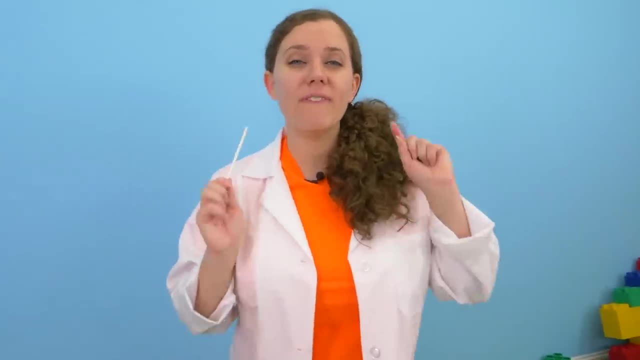 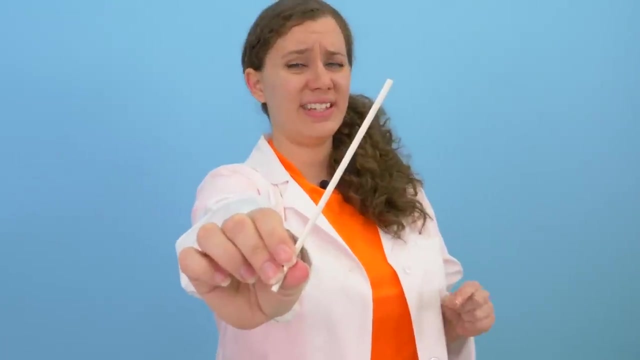 the best, and it's also on a stick, so it's easy. the first thing that we're going to do is build the very center for our rock candy. now we are going to use these paper sticks- mm-hmm paper sticks. you don't eat the paper stick. it's kind of like what would be in the center of a lollipop. 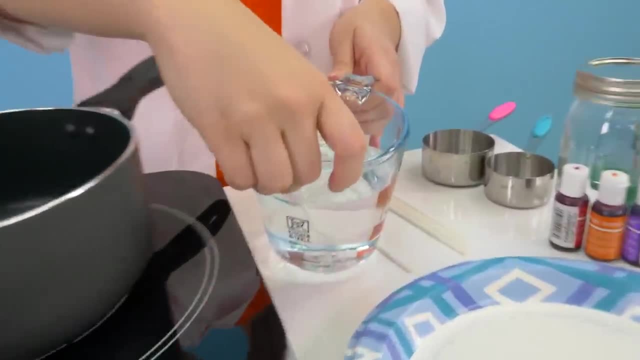 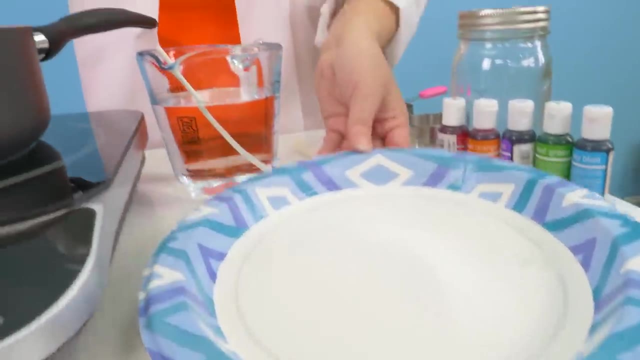 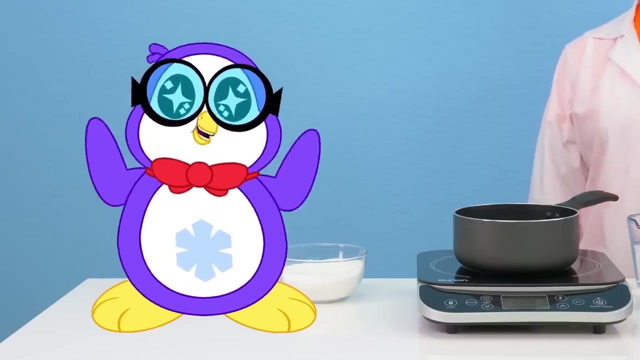 we're going to take the stick, we're going to dip it in water and we're going to pour it in the container water like this. uh well, we need sugar too, Definitely need some sugar. So let's get some sugar on a plate. Perfect, Yay, Sugar, Woohoo Sugar, sugar, sugar, sugar, Yeah, sugar, There's. 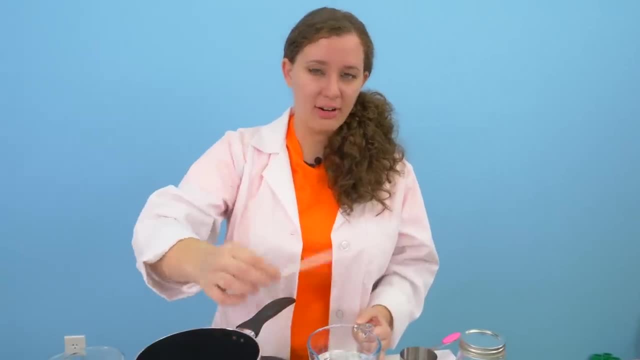 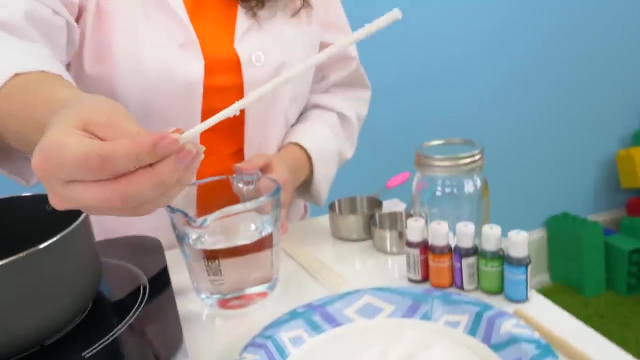 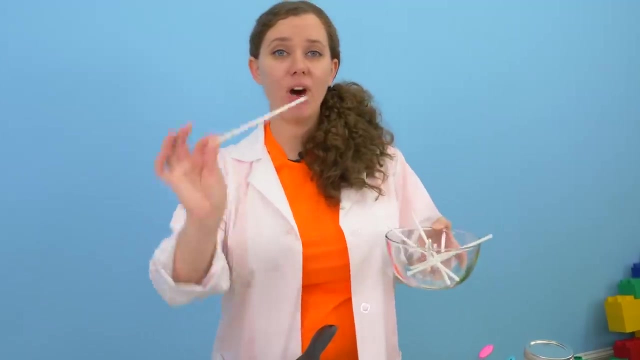 going to be a lot of that. Now that we have our stick all nice and wet, we're going to roll it around, get some sugar on here and it should look something about like that, which this will give our rock crystals plenty of stuff to grow on, Now that we have all of our sticks coated in sugar. 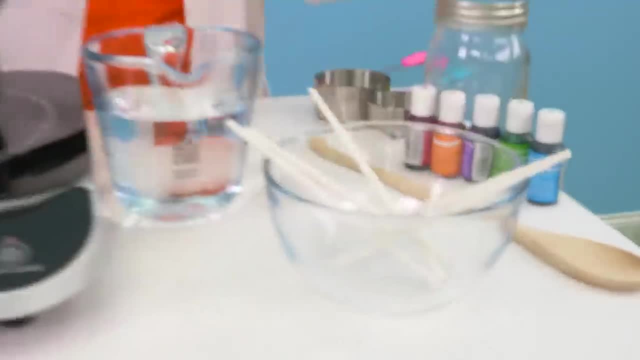 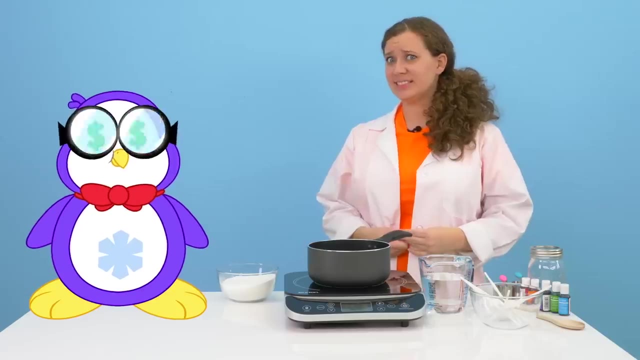 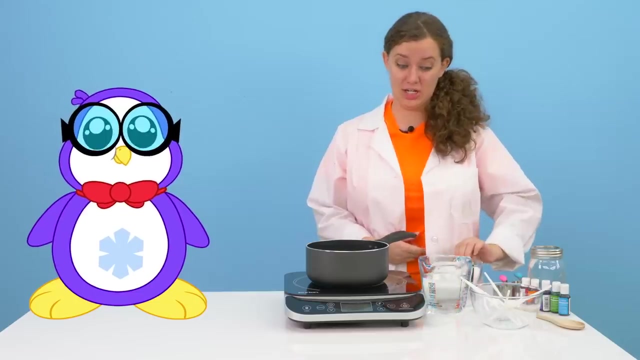 we're just going to set them aside and let them dry so we can use them later. Now we can commence with the creation of our rock candy. Uh, that's right, Peck. Uh, maybe I should just take this sugar away and put it over here. So the first thing we're going to do is add water. We are 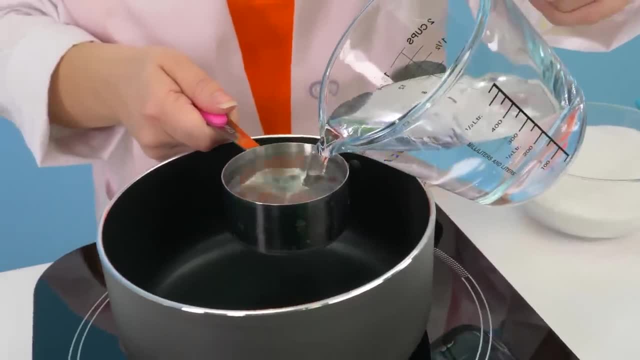 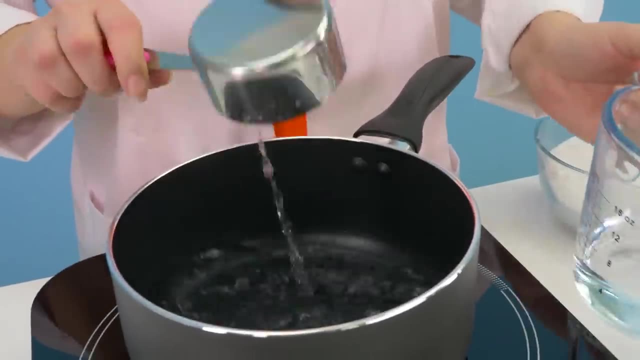 going to add water- One cup of water, which all I could find was a half cup measuring cup, so we need two of them. Then we're going to turn on our cooktop and we're going to turn it on boil so we can get it cooking. 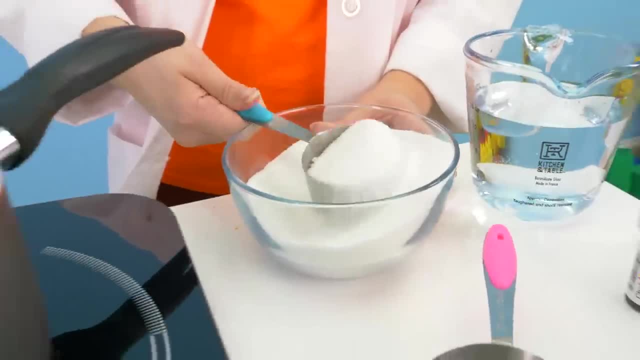 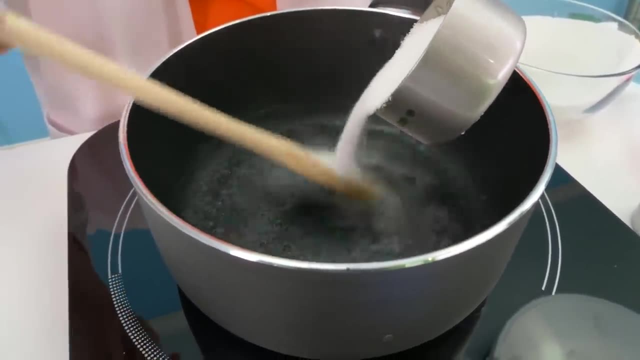 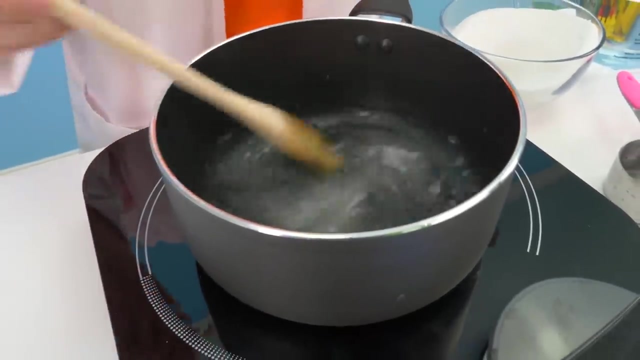 Ah, bubbles. Now we're going to add our sugar. We're going to slowly mix it in, We're going to try to use about two-thirds cup and we're going to make sure it dissolves fully in the water. We have a bowl of sugar water now. What are those jars for? 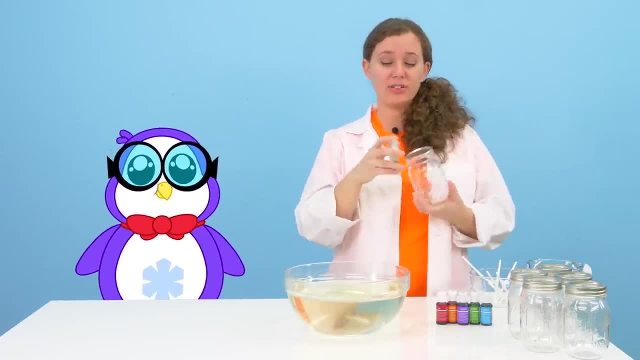 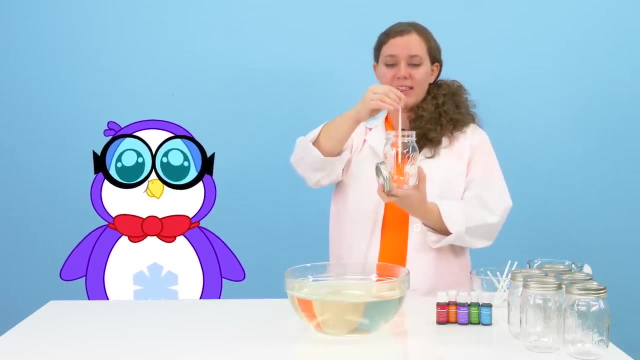 Well, that is a good question, Peck. We are going to use all these different jars to grow our individual rock candies. Now, we don't need the lid, because this is actually going to go in here just like that and grow all of our crystals. 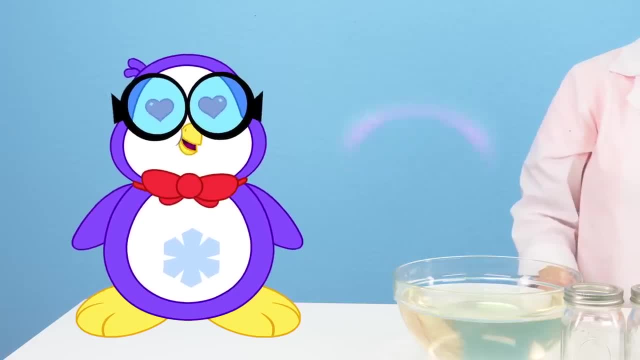 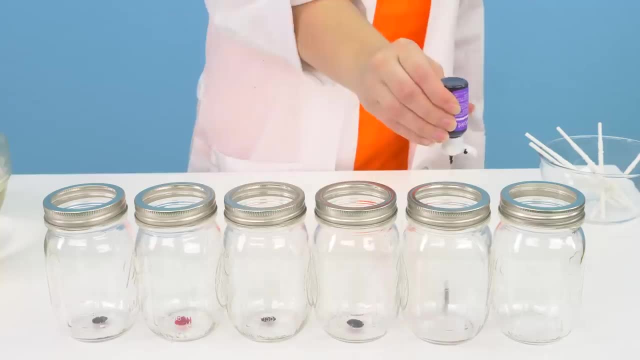 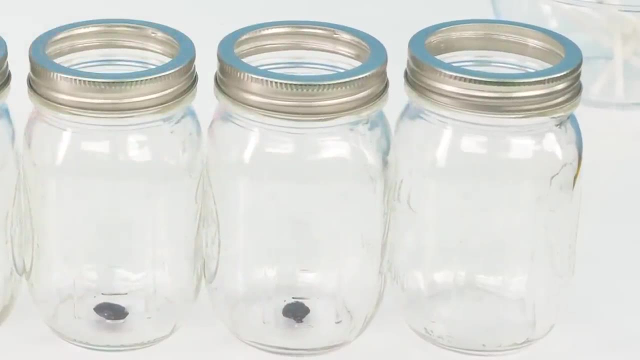 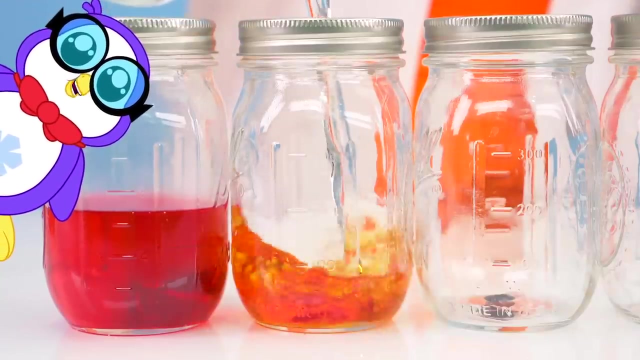 Red, orange, green, blue, purple, And I think I'm going to leave the last one clear, because I just want to see what the regular rock candy looks like. Red, like Red Titan, because he's super red. Orange, like Moe- He's so crazy. 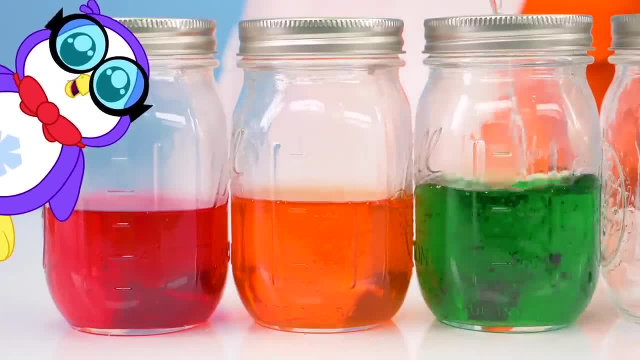 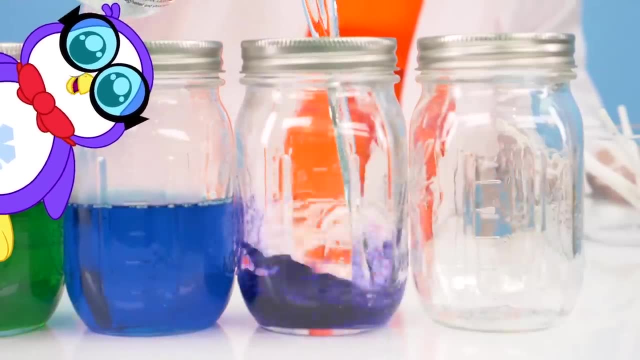 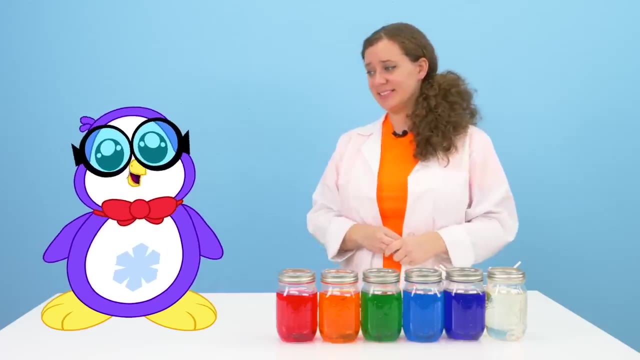 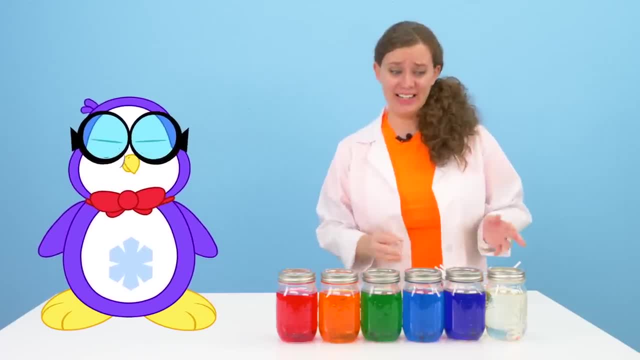 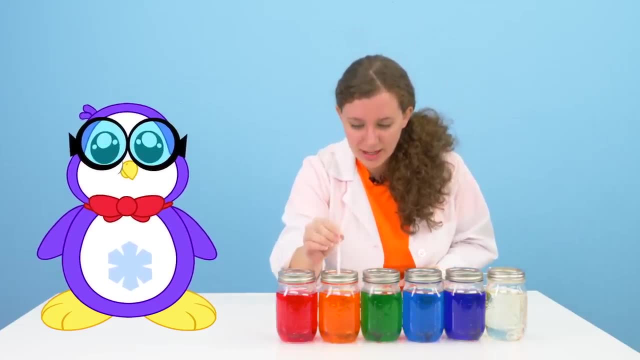 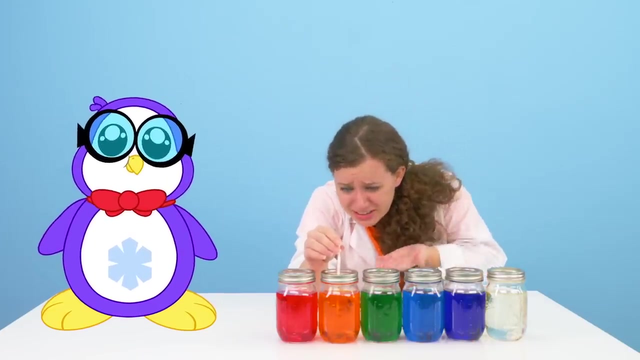 Wow, Peck, that was really something Moving on. the last thing that we have to do to make our rock candy is we just take the center piece, our sugar sticks, and then we just put them right in the center and wait. we need to hold it in place and well, I don't have six arms and if I let it go it's gonna. 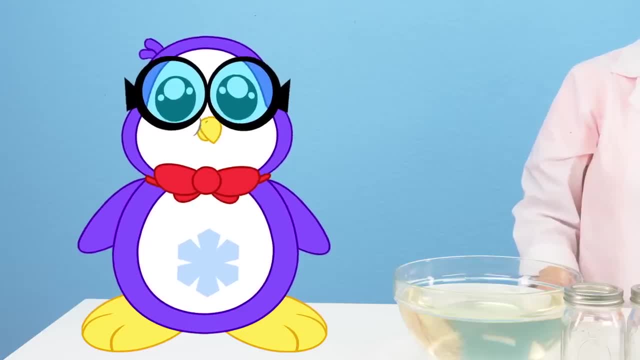 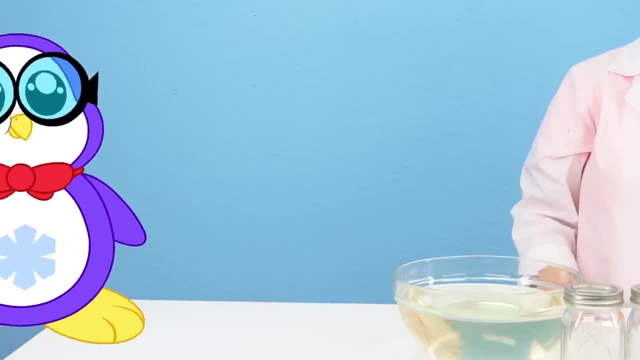 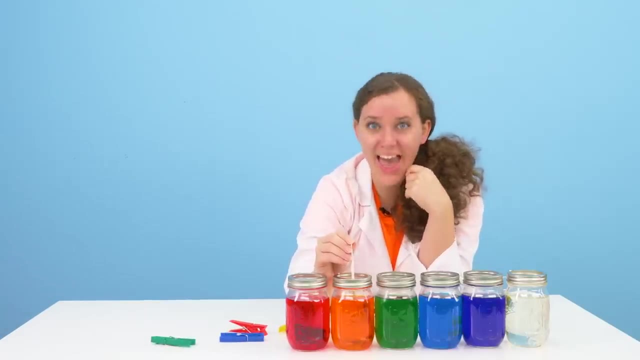 it's gonna fall and oh no. Oh, don't worry, Bree, I know what we can use. Okay, Peck, hurry, Be right back. I sure hope Peck gets here soon. I'm getting so tired. Hey, these are perfect. Oh, that is much better. 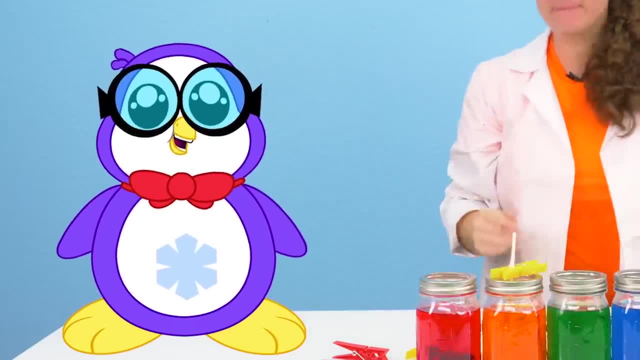 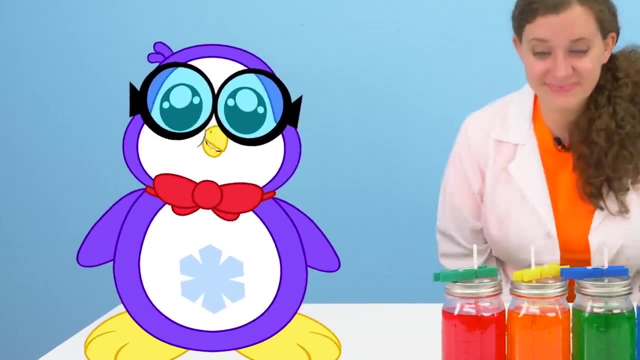 It was a success. now we can start making the candy. Hmm, hmm, hmm, Hoo-ha. Oh, that's awesome, Oh, that's awesome, Oh that's awesome, Ha, ha, ha, ha. yeah, How long do we have to wait? Like five minutes. 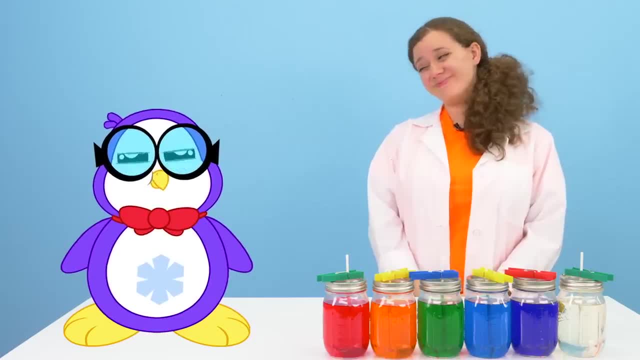 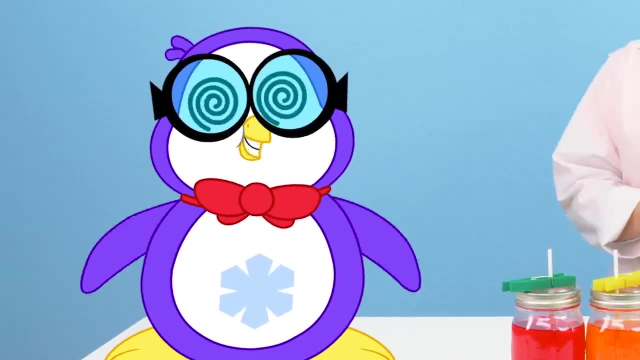 Ha ha, oh, I mean ten minutes. Hmm, Thirty minutes. No, Peck it's. it's gonna be more like five days. Five days What, But? but that's like 7,200 minutes, Noooo. 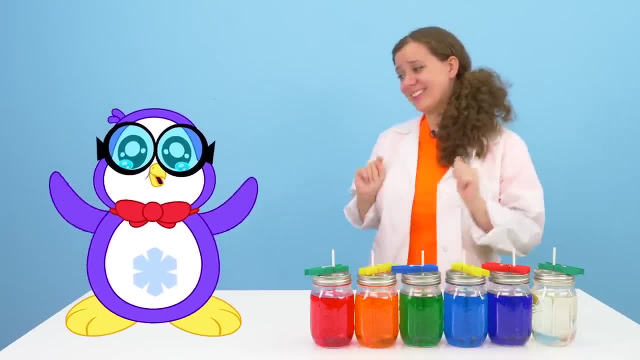 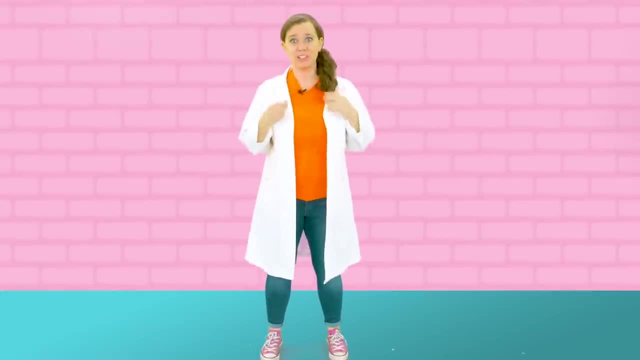 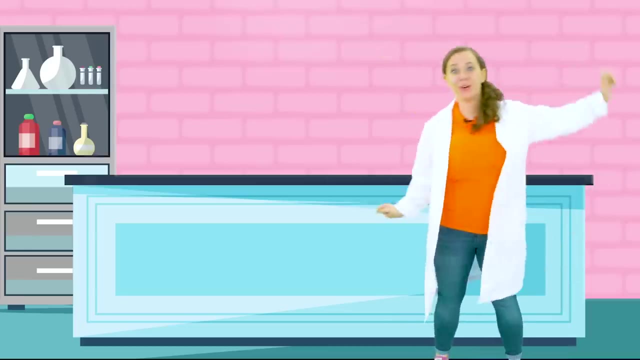 Okay, uh, I'm just gonna go. Don't worry, Peck, you got this, I'll see you in five days. Bye, What? Ha, ha, ha, ha. well, since we're just waiting here, how about we take a look at the science behind rock candy? 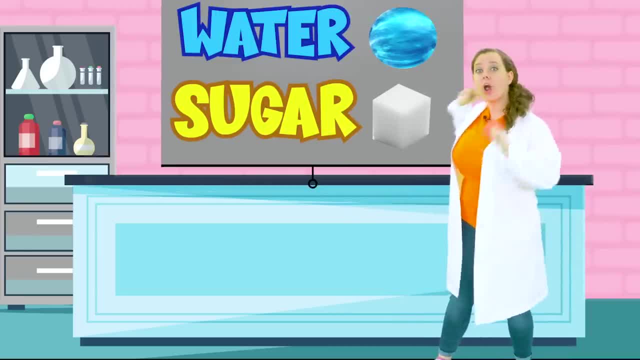 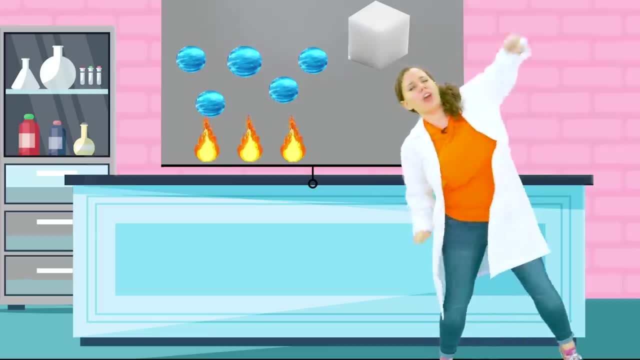 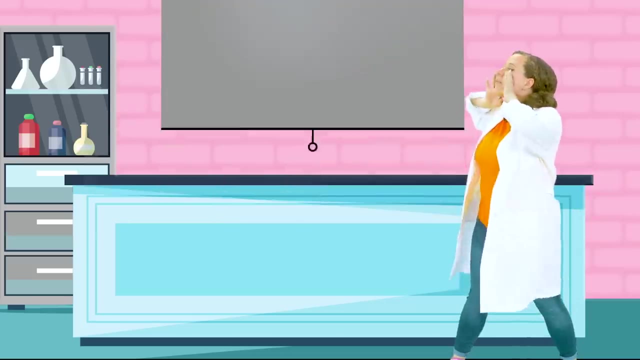 So water and sugar are both molecules. Now, when we heat up the water, the water molecules spread apart And then we're left with all this space that we can add a lot of sugar to. Hey, bring in the sugar, Bring in the sugar. 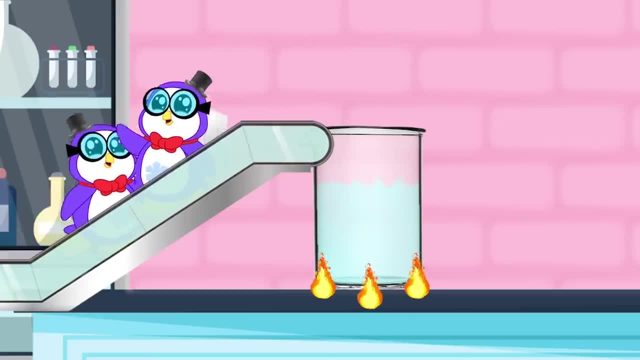 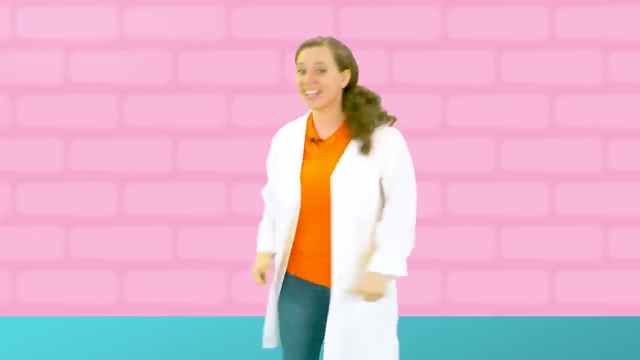 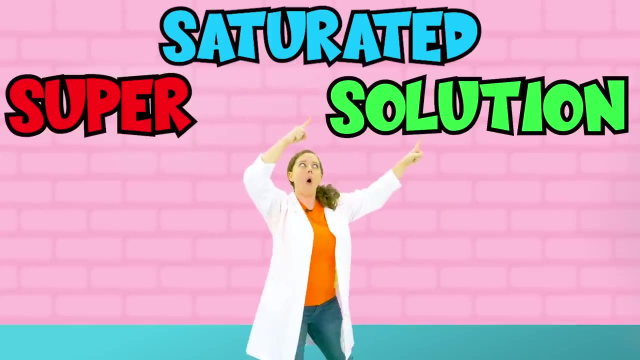 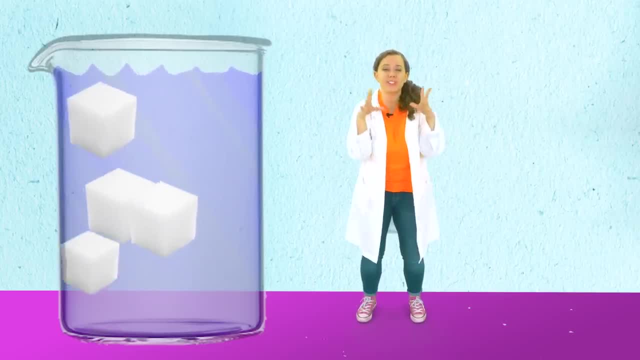 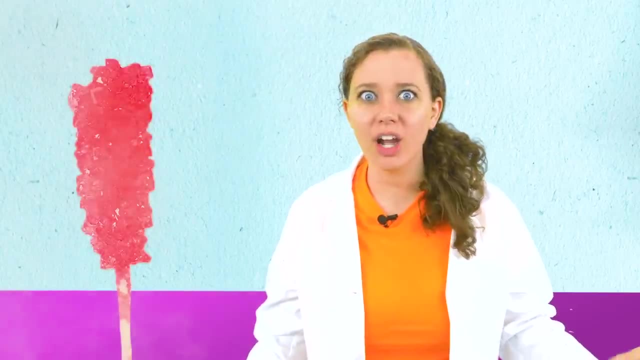 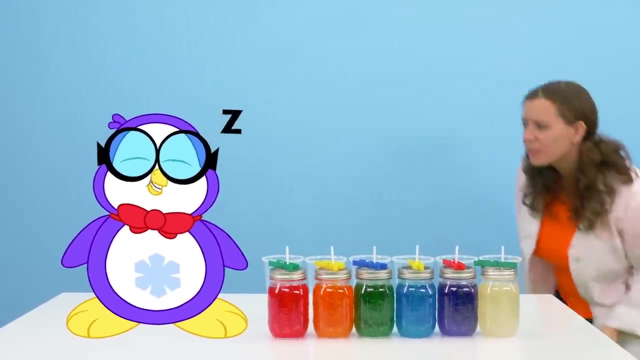 As our solution cools, the sugar begins to crystallize, And these crystals form rock candy. Speaking of rock candy, I think ours is ready. Let's go. let's go, Mmm candy, Mmm sugar Peck. 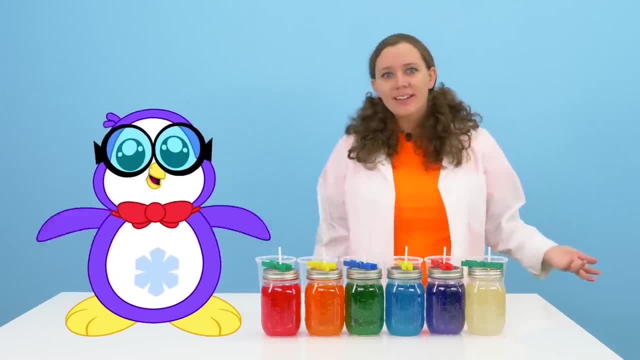 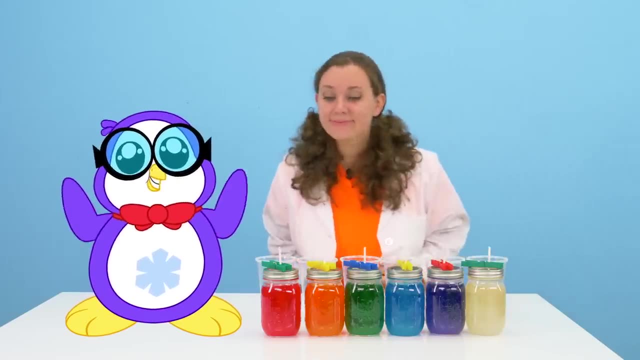 Peck. Whoa, has it been 7,200 minutes? It has, which is why I'm here. It's candy time. Candy, candy, candy, yeah, But but how are we gonna get the candy out? 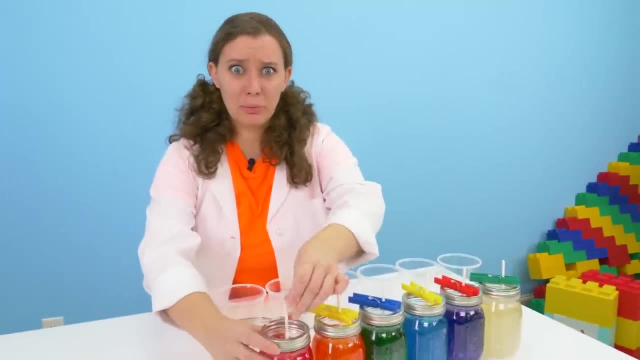 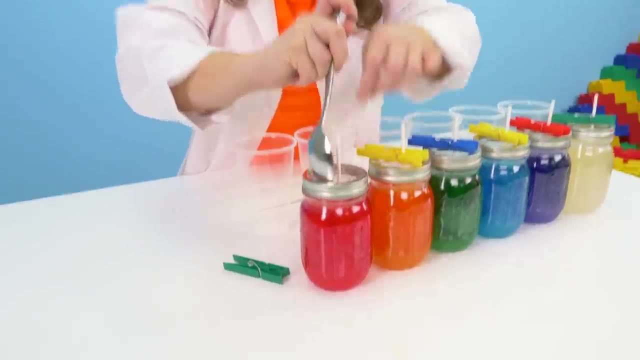 You're right, Peck. You're right, Peck. these are stuck in pretty good, But I think we can use this regular plain-jane spoon to maybe chisel it out. So we need to break the top layer. Oh, oh, my goodness. 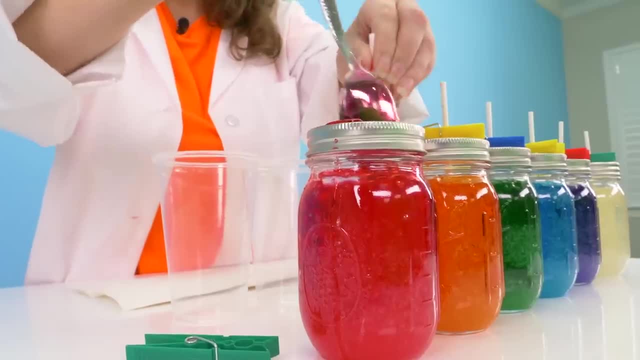 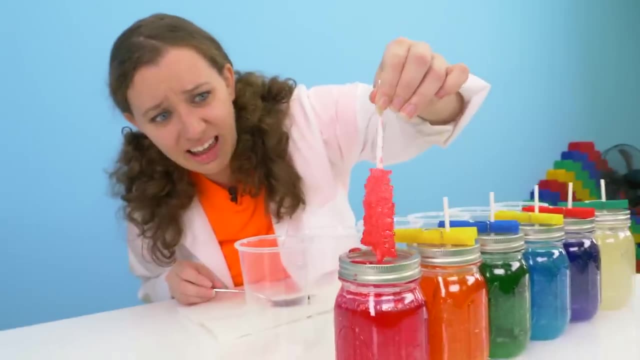 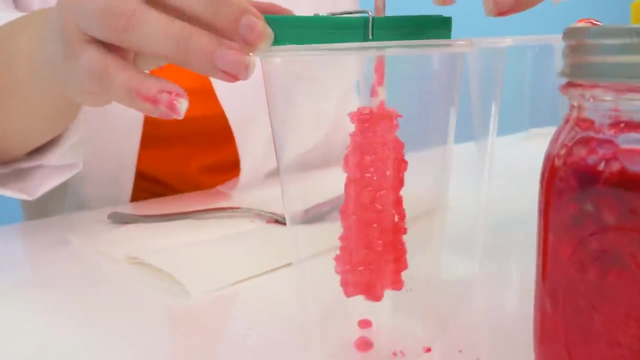 That is a lot of sugar crystals. Whoa, there we go. Oh man, it is all sugary and sticky and yummy. We definitely need this to dry. So we're gonna use this cup to let our rock candy dry, so it collects all this really sticky stuff and we don't make a mess everywhere. 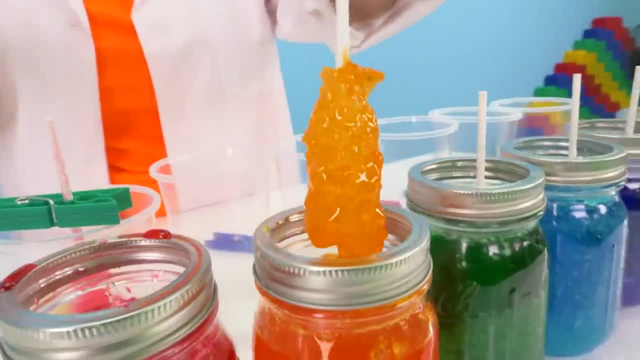 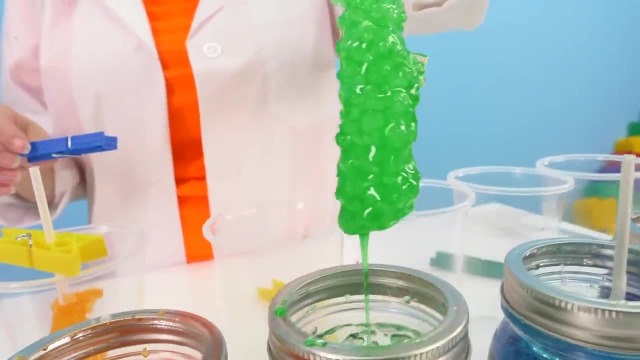 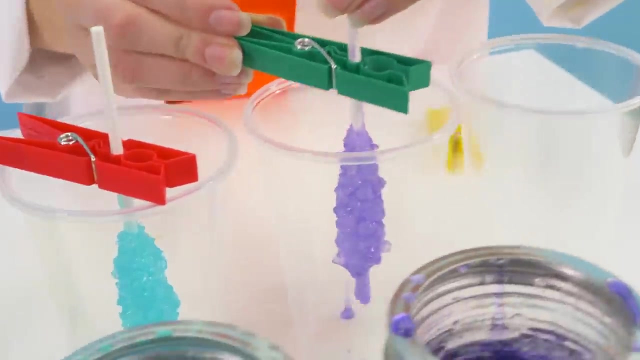 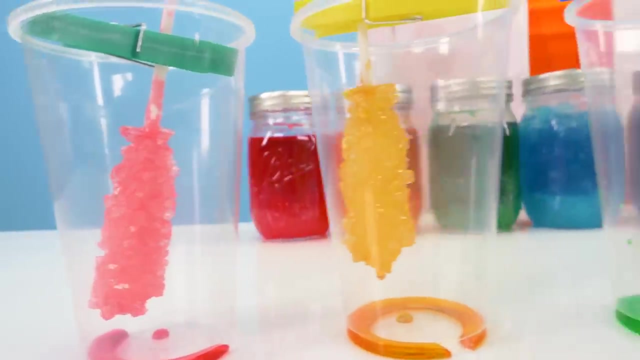 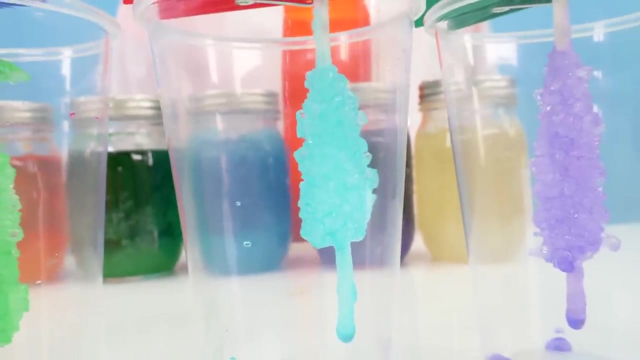 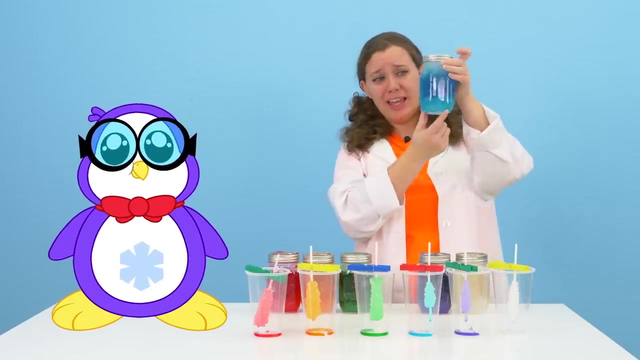 Oh wow, it looks so tasty And crunchy. Phew got it. Oh gosh, I can't wait to try some. Mmm, mmm, Wait a second. that blue one looks broken. What happened? Well, Peck, the stick got stuck in the jar when I went to pull it out, and that's because it was a little too close to the bottom and all these crystals grew around it. 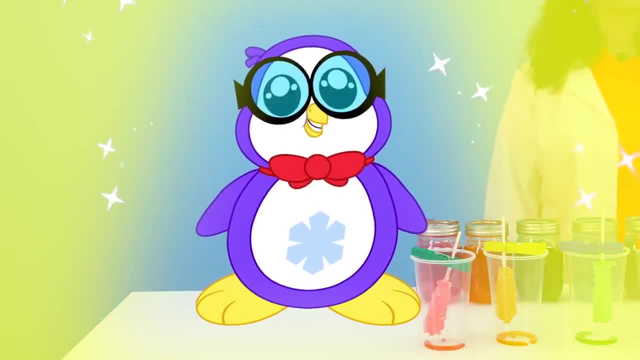 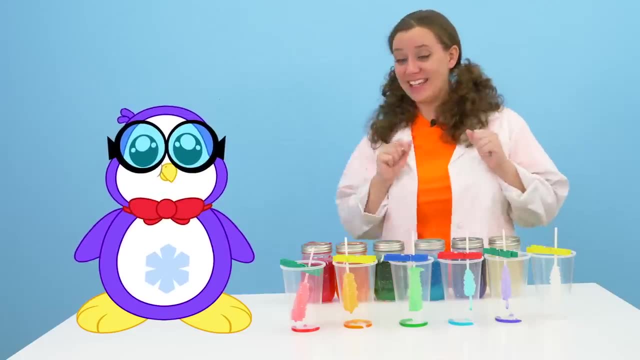 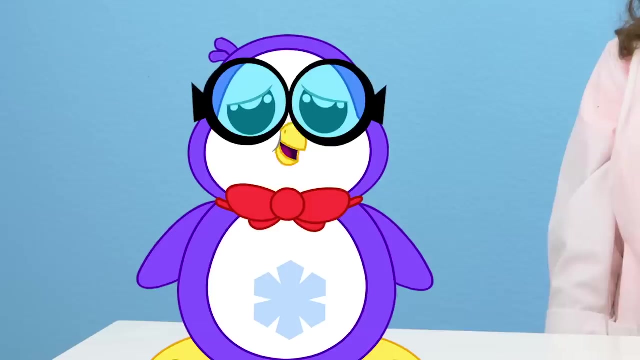 Um Brie, is it okay if I try some of the candy now? I've been so patient and helpful. We can definitely eat all of this rock candy Really As soon as it dries, Oh, Mmm, mmm. 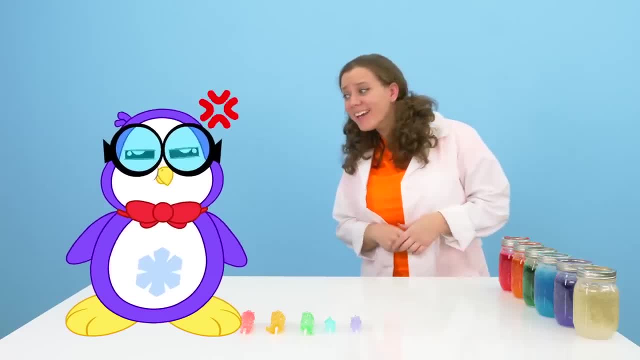 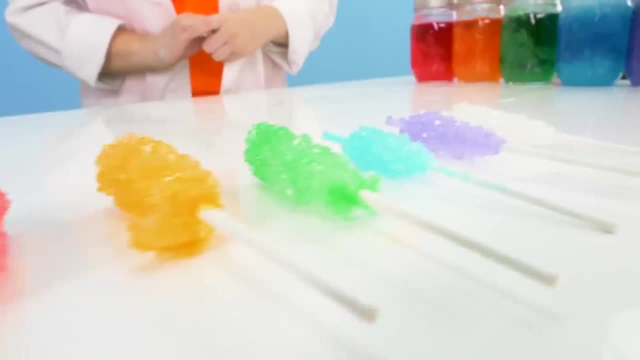 Oh gosh, I can't take it anymore. Peck, Huh, The candy's ready. My patience finally paid off. Uh yeah, sure, Good job. Peck, Now is the best part We get to taste test. 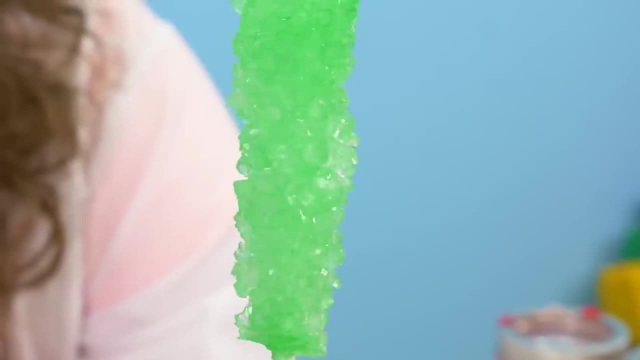 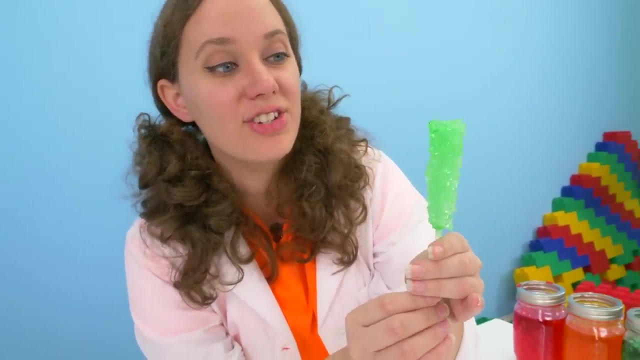 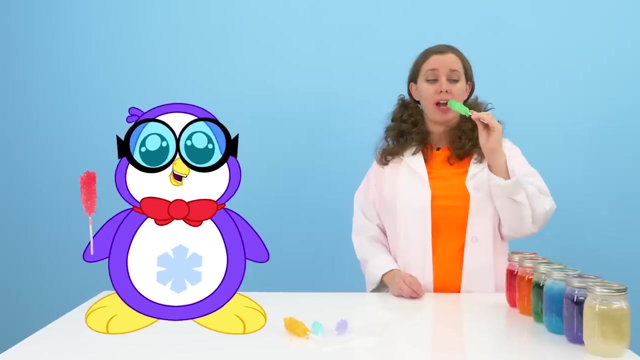 Ooh, Ooh, Ooh, shiny. Look at all those crystals. They are so yummy and shiny. And the best part, Mmm, that is really good. Mmm, this is so good, It's filling me with energy. 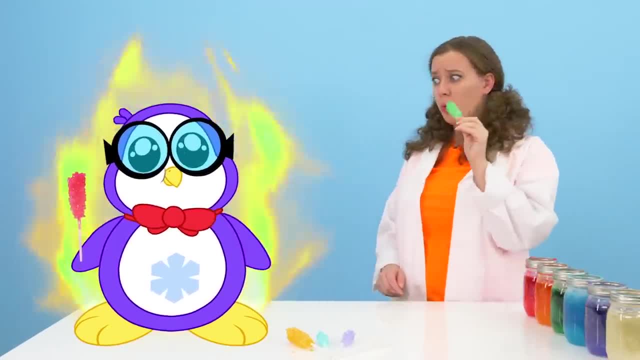 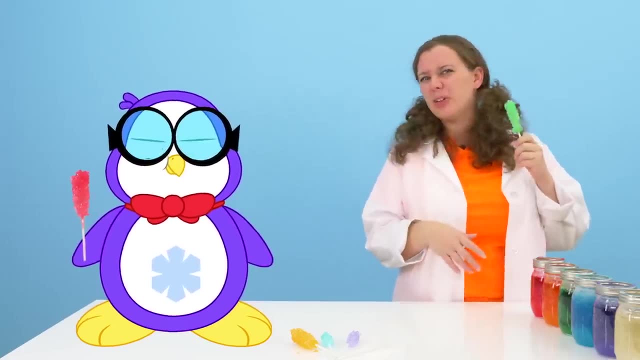 Whoa. And the best part about this is it's so simple to make. You can make it at home too. It just takes a little bit. It takes a little while. Yeah, I'm going to eat the rest of them. 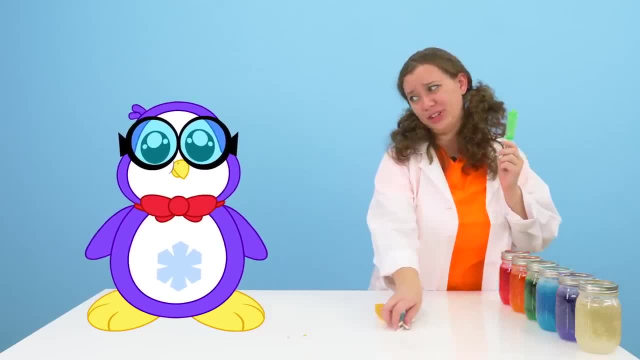 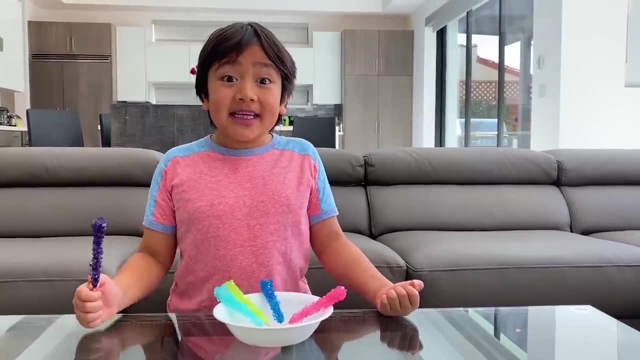 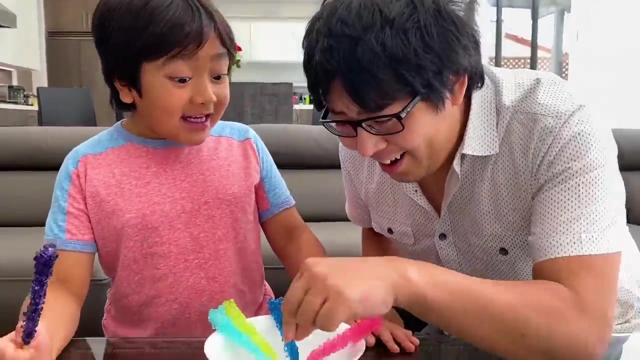 Uh, maybe we'll save those for later. Peck- okay, Thank you for showing me how to make these rock candies Peck. It's so cool. Oh, look at those. You want to try rock candies? Yeah, I picked the blue one. 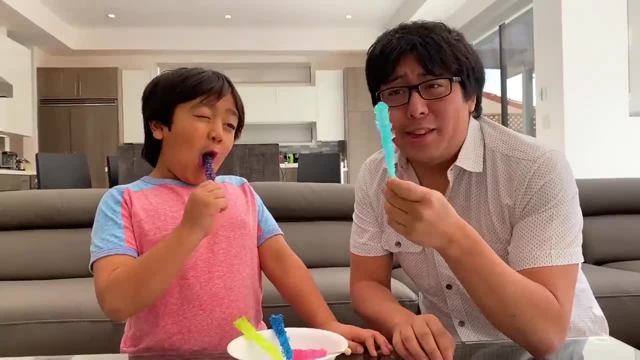 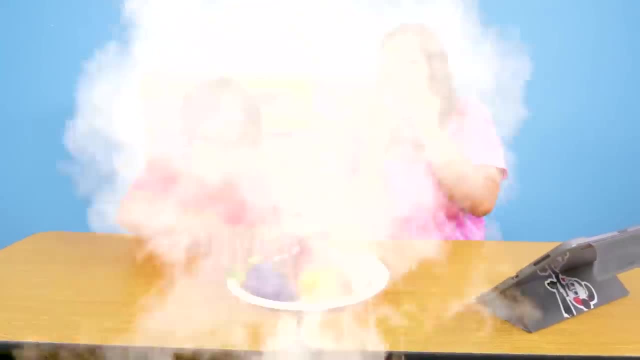 Oh, this is so cool And it tastes great. Oh, it's so sweet. Okay, guys, I can't wait for snack time. Whoa, A plate of fruits. Ooh, This one is fun. Okay, Well, I like carrots. 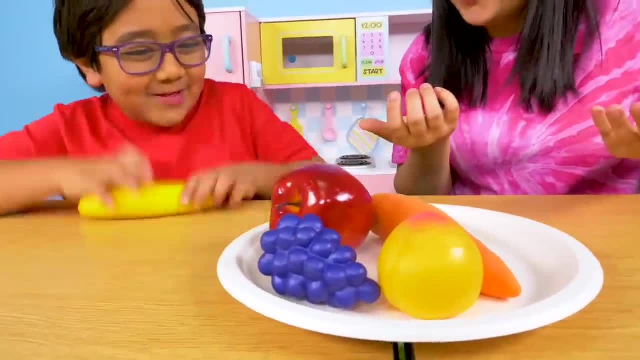 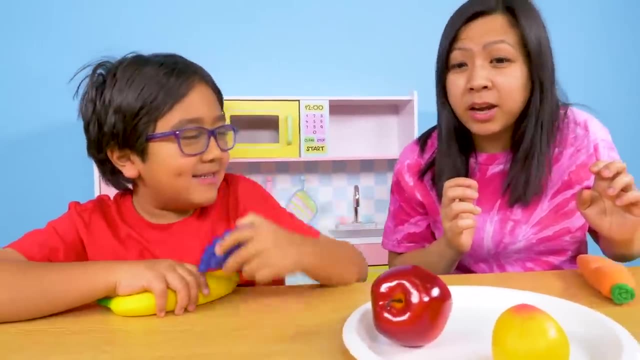 They're good for your eyes. Well, I'm going to pick grapes. Okay, Well, I like peach. There's only one left. Hmm, Oh, No, They're not yours, They're mine. Oh, Oh, Oh. 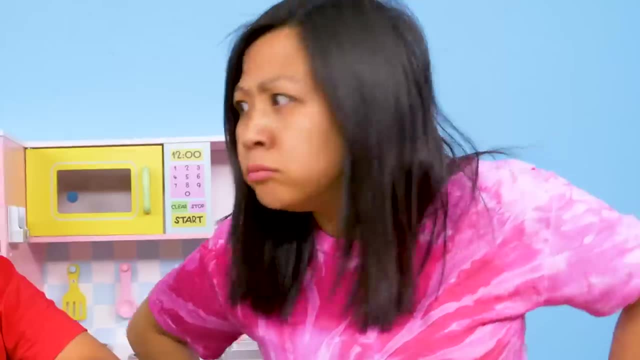 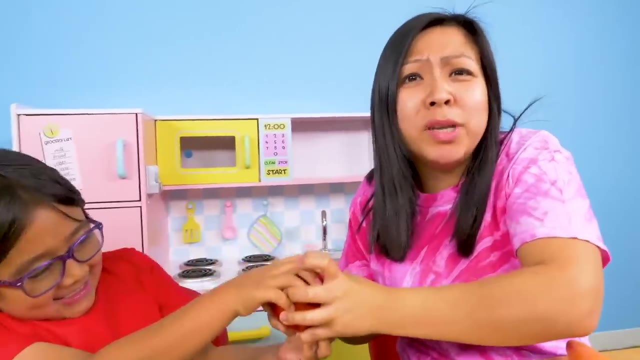 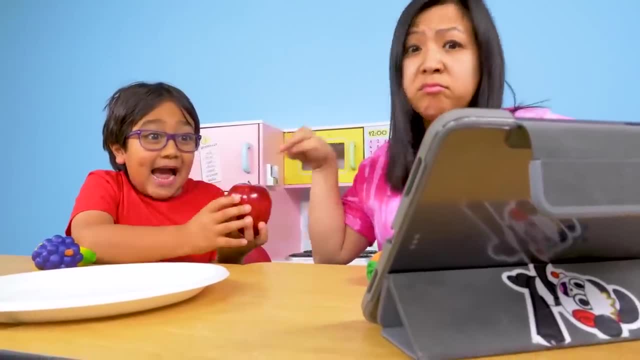 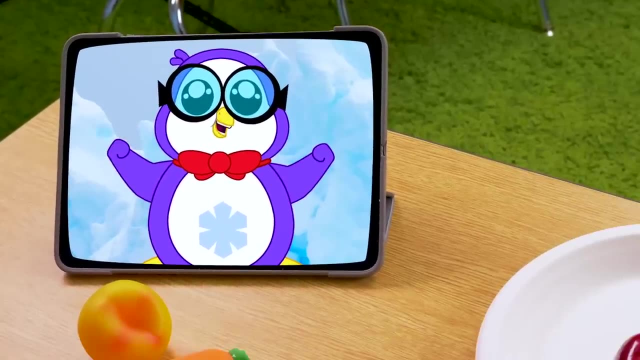 It's probably going to be me The last apple. Hmm, Oh-huh, I have an idea. I will build a rock paper scissors machine for you, And then the apple will go to the winner. Okay, Peck. 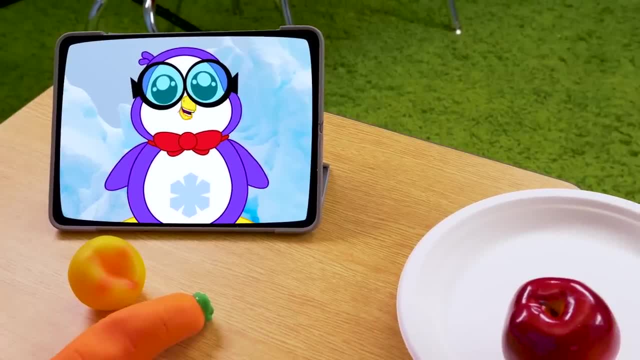 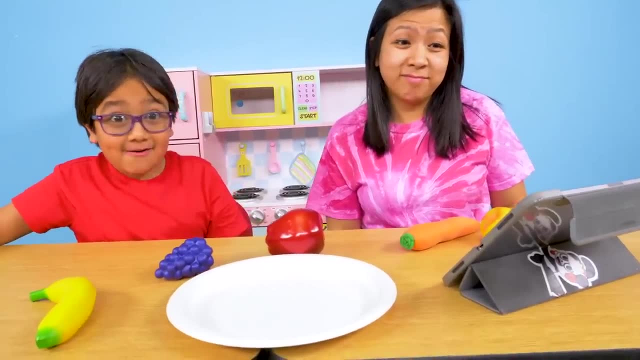 I can't wait. Don't worry, I got a good idea. What is it? Oh Okay, Peck, I can't wait to see how this machine you're talking about is gonna look like. Hey Ryan, we have to wait. 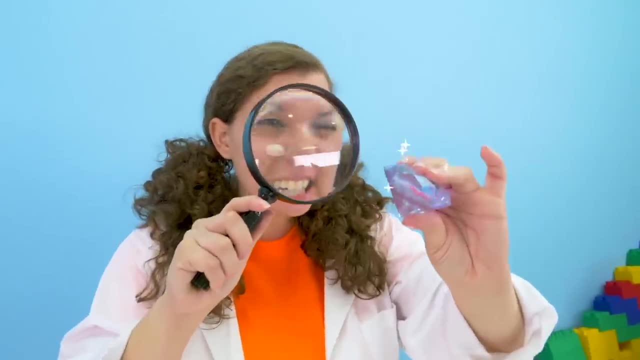 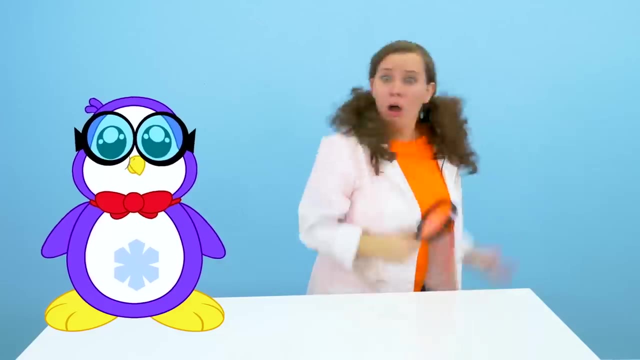 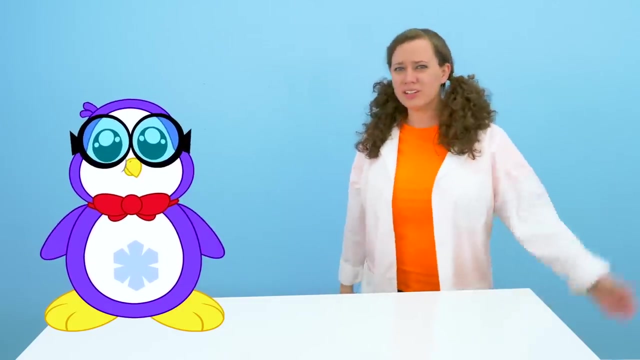 Whoa with this color and how shiny it is. this thing has gotta be worth so much money. Ooh, We got another experiment: to build Peck. Wait, what about an experiment? It's time to build a rock paper scissors machine. 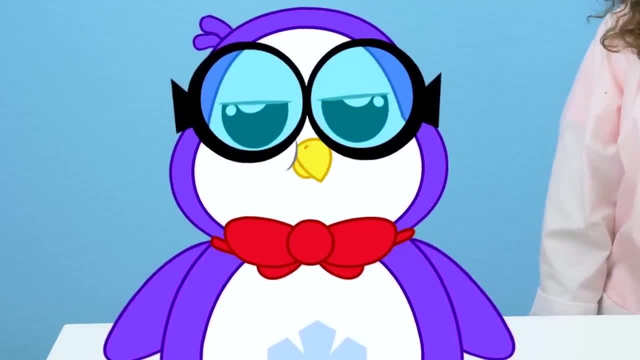 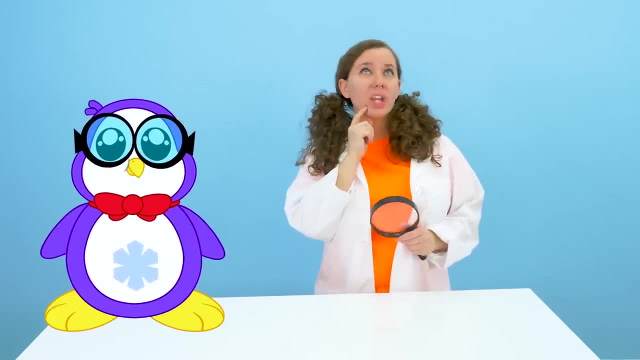 A paper rock scissors machine. Hmm, it's rock paper scissors, but yeah, do you know how to build one? Hmm, well, a paper rock scissors machine could be pretty cool, but we're gonna need a lot of materials. 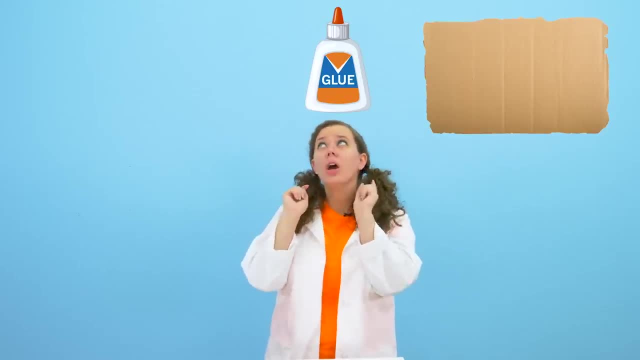 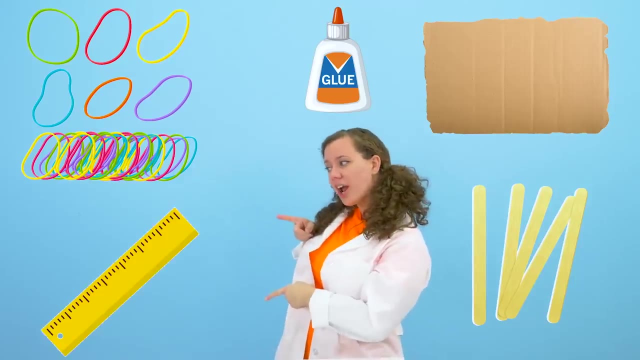 So we're gonna need things like cardboard, glue, rubber bands, sticks, and straight lines are always fun, so we definitely need a ruler. That's a really long list. So, with the stuff, where are we gonna get all this from? 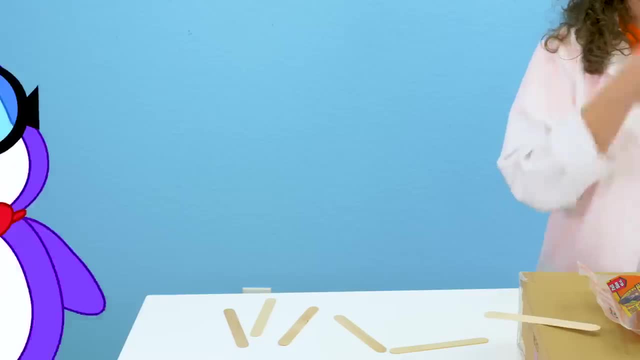 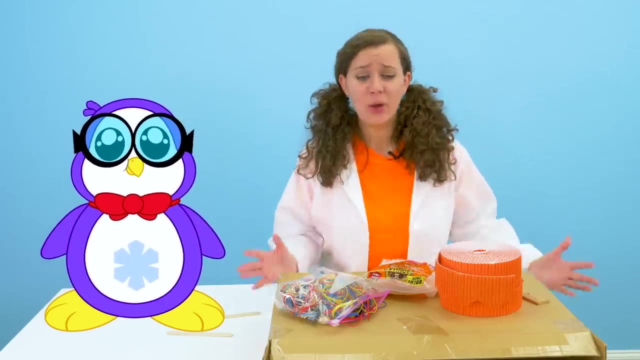 Whoa, that's everything we need. That's convenient. Yeah, I got all the stuff. Now what do we do? Whoa, great job. Peck Now to get started. we are gonna use this box. We'll get that later. 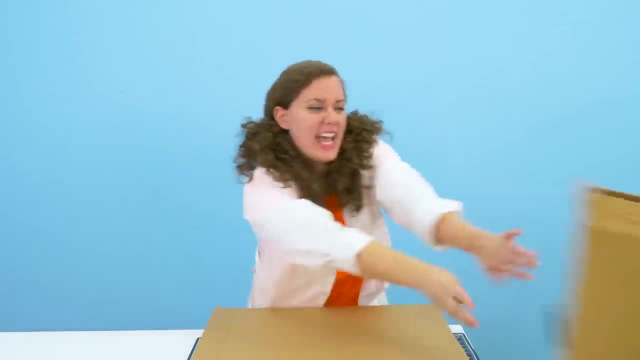 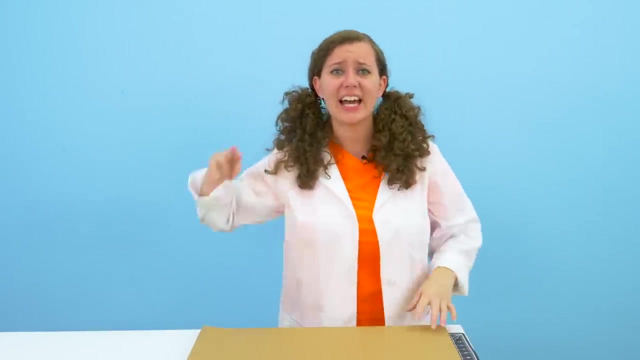 Now we're gonna cut up our cardboard, which will give us something flat like this, And with this we're going to trace and cut out all of our shapes. First, we're gonna measure and draw all the pieces that make up the outside of our machine. 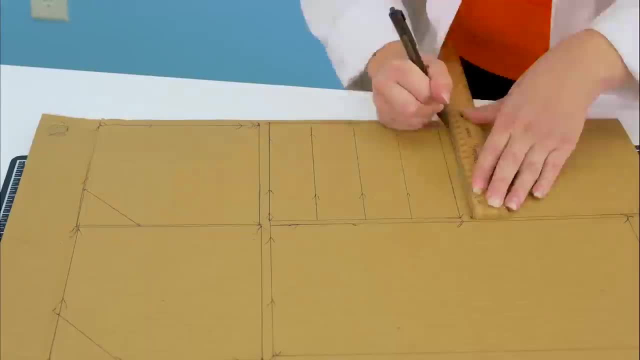 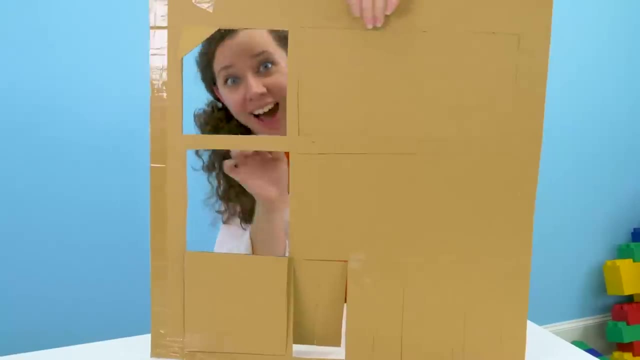 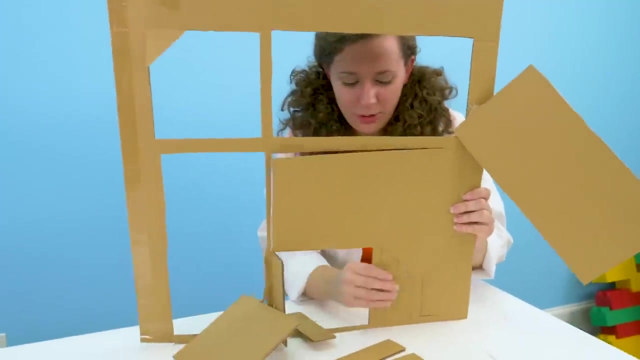 Once we finish that, we have to draw all of the little ones that go on the inside. Now it's time to punch out all of our parts. Let's see, Oh, Oh Well, it's kind of working: Bink, bink, bink, bink. 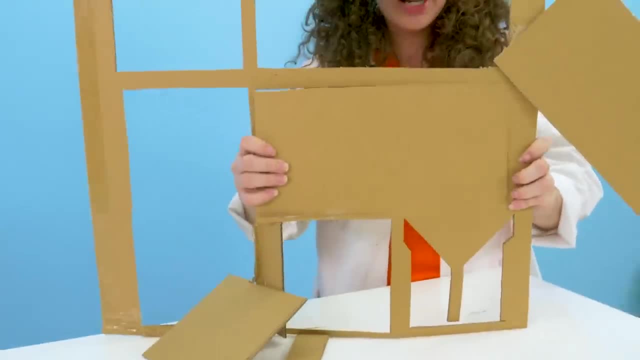 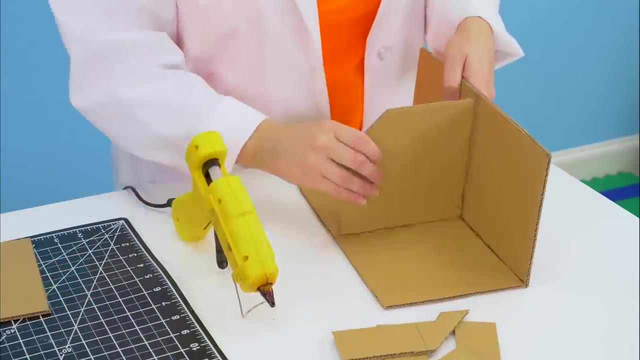 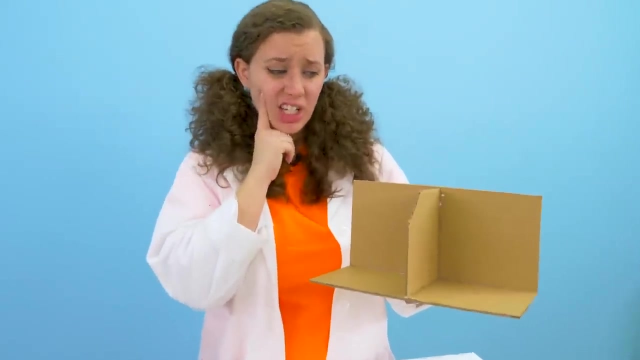 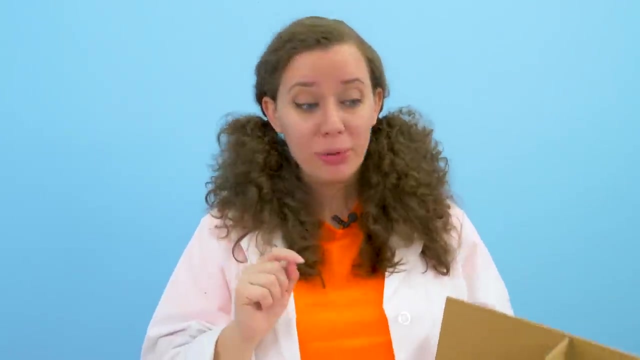 Ah, and one last one. Well, Let's start gluing the pieces down. Hmm, You will need an adult's help for this part. It looks really good, But now we need the little spinny tubey thingies. Oh, Those are called the reels, but you know, I think I have the perfect idea for the spinny tubey thingies. 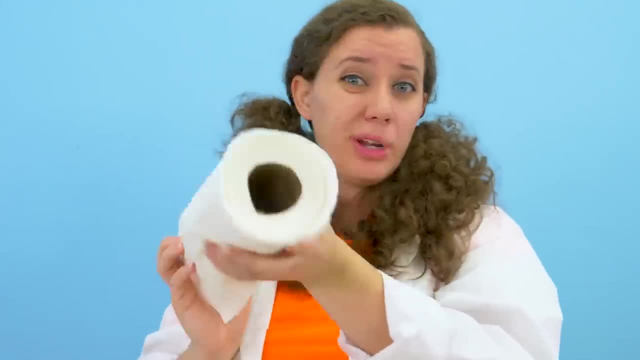 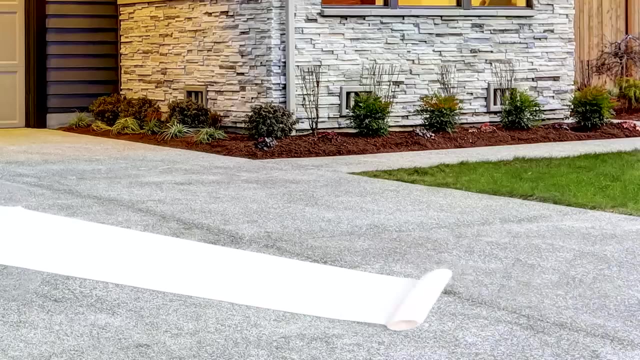 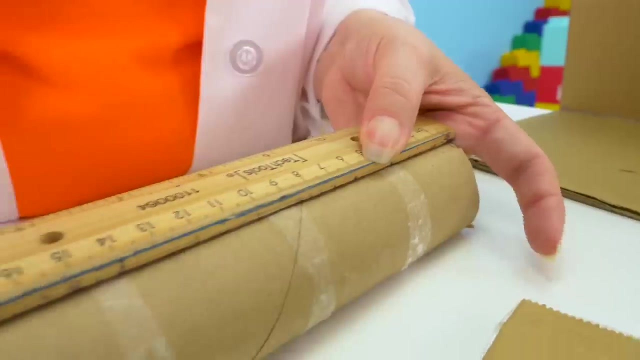 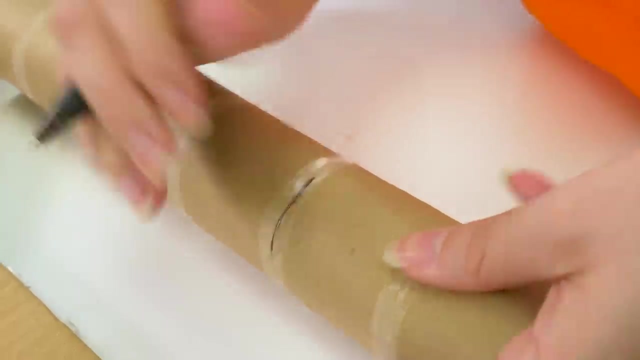 I think we could use this roll of paper towels. It's already pretty much shaped like it, But I'm gonna get all these paper towels off. Oops, We want our reels to be the exact same size, So we're gonna measure very carefully And we're gonna make sure we cut straight. 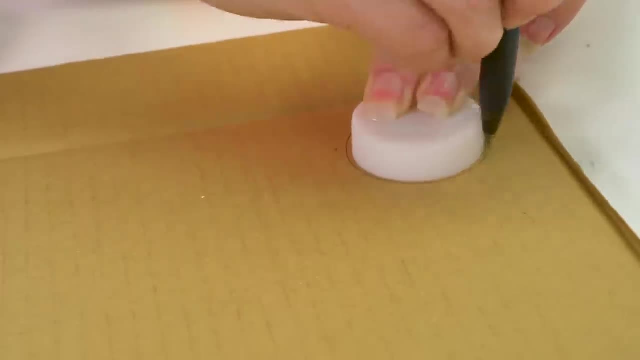 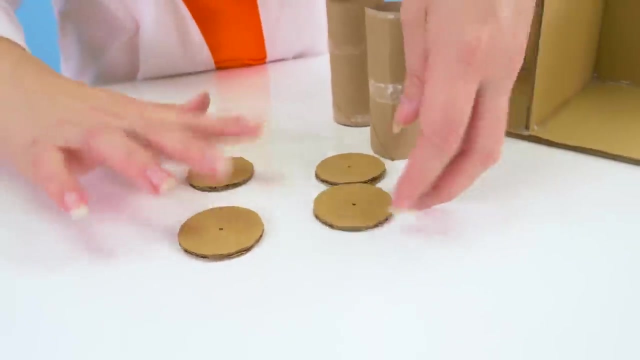 Whoo. now that that's done, We just have to make our circles. I found this cap lying around and it's the perfect size. Oops, all right. Well, we have all four of our circles now We just have to put them in here, and then we're just gonna glue it into place. 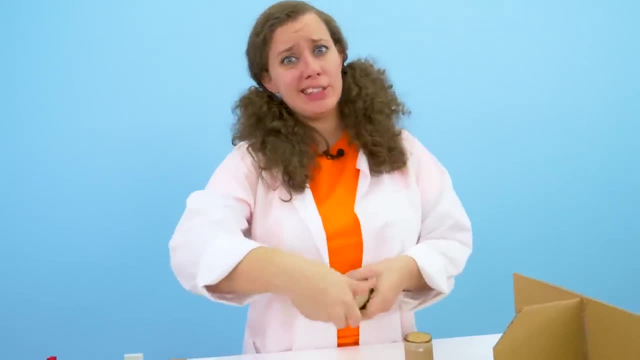 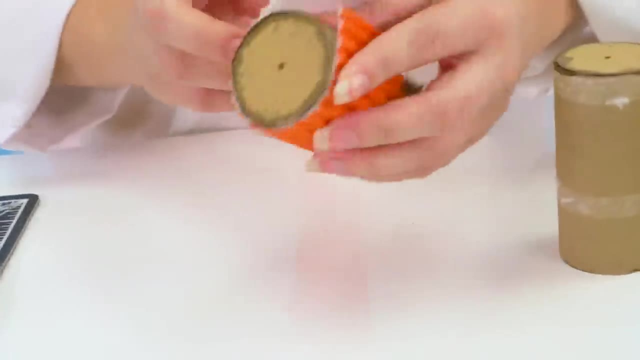 That looks good and dry. It's nice and strong, but we need something to help our reel spin like that. I have the perfect idea. We're gonna use this really pretty border paper. We're gonna wrap it around like this, and I think that's gonna help a lot. Let's get started. 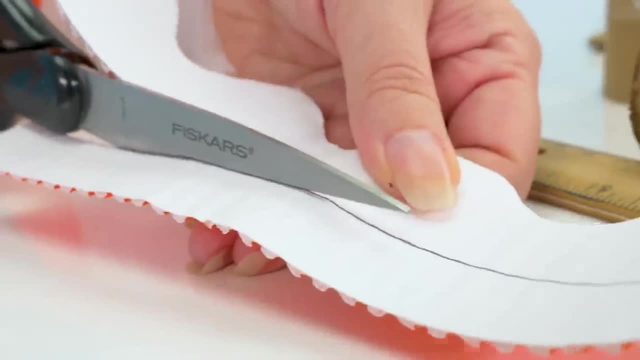 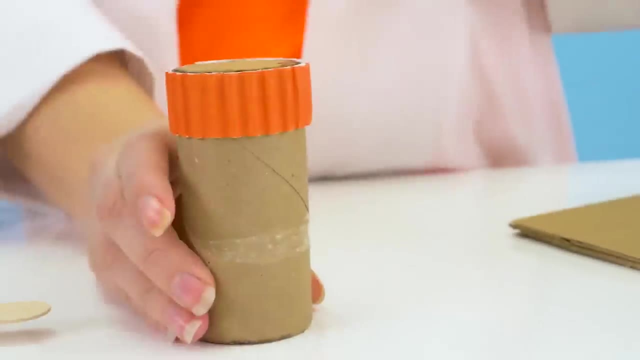 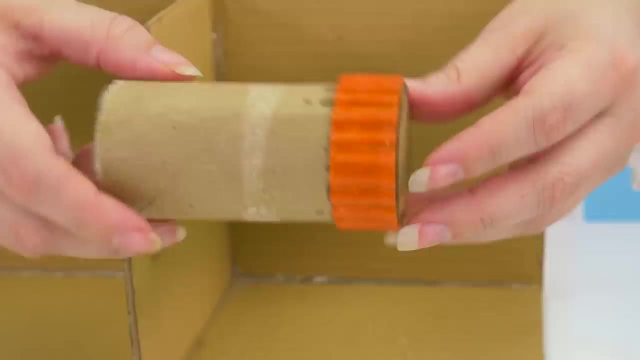 We need to measure and cut our border paper. Once we cut it Nice and straight, then all we have to do is wrap it around our reel and glue it in place. We have to glue up the orange gears so they can become extra sturdy. Ha ha, All right. Now everything is nice and dry. Our fingers aren't sticking to it. It's nice and hard. 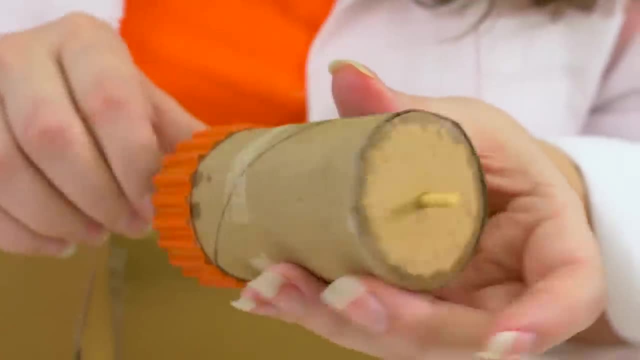 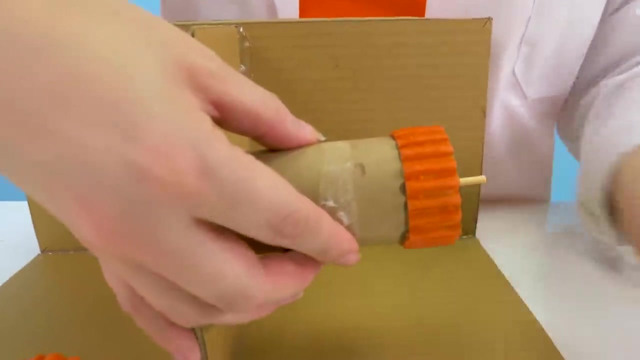 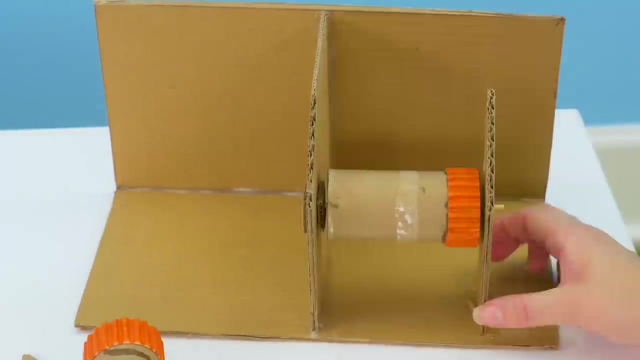 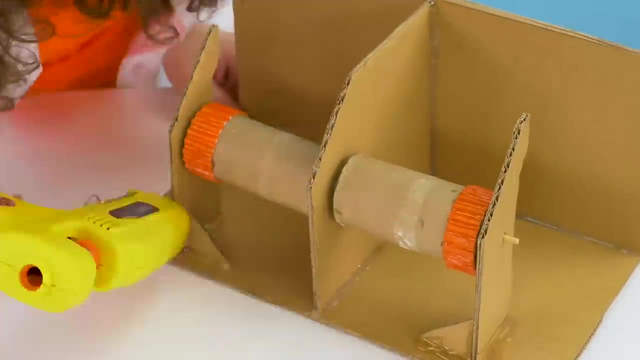 We're gonna take our stick and we're gonna try our best to get it all the way through. Now we just set it in place in our machine, Put the other side here to hold it in and we just glue this guy together. Now this part can be very tricky. You need to leave enough space for your reels to spin, but not too much space, or they'll fall off. 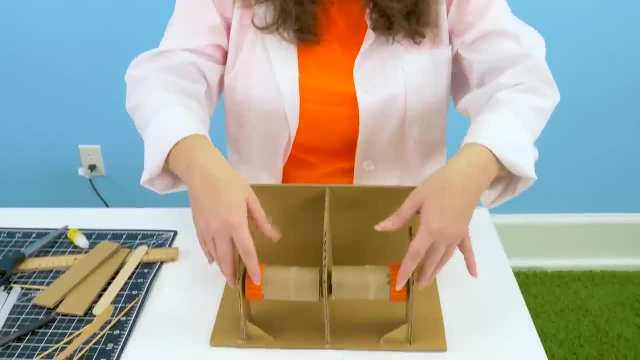 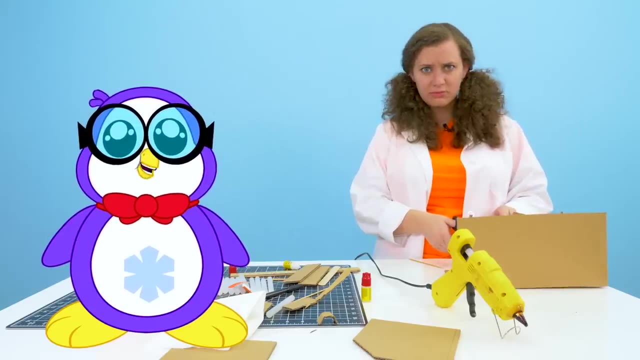 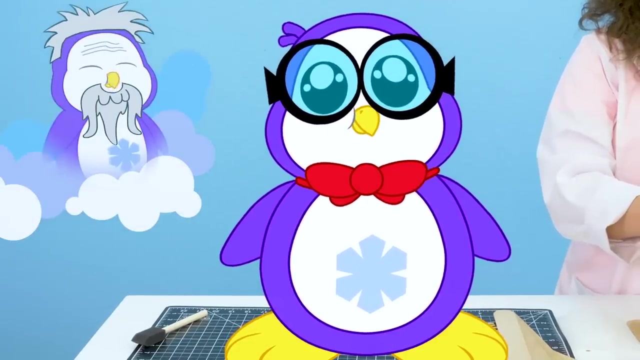 So, after everything is glued into place, you should be able to do something like This. ha ha Yes, soon My plans will be complete. I'll be finally able to win in rock-paper-scissors. For generations, our family has only been able to throw paper. 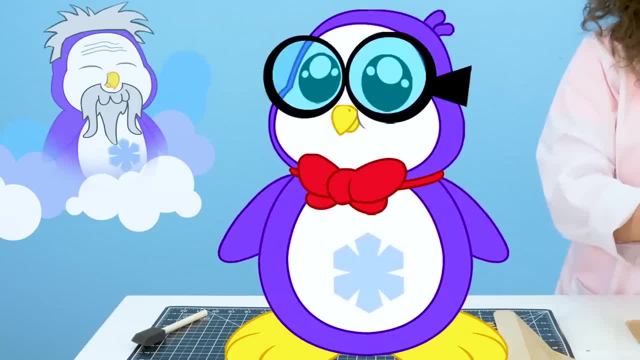 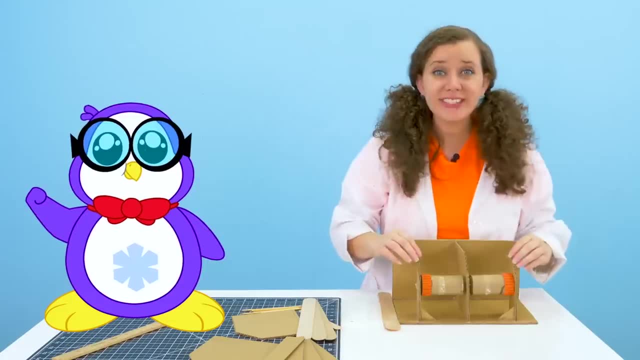 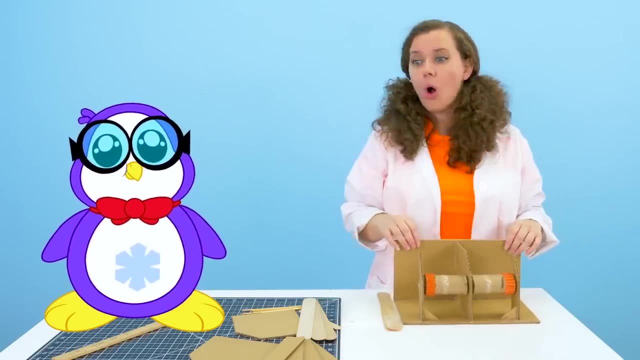 But with your smarts, Peck, I think you'll be the one to be able to change our fate. Looks like all the glue is dry and it's spinning- great. Looks like it could use a lever to help make it spin. These giant popsicle sticks are gonna work great. Thanks to Peck. 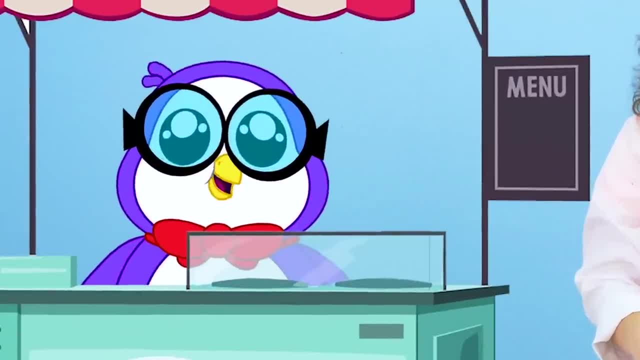 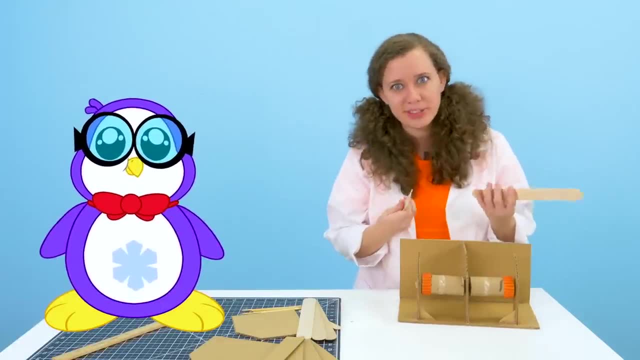 Yeah, feel free to stop on by and check out Peck's channel for more videos like this one. Come by Peck's premium popsicle stand, where we sell discounted popsicles at premium prices. Yeah, yeah, um. the only thing about these popsicle sticks are they're a little. 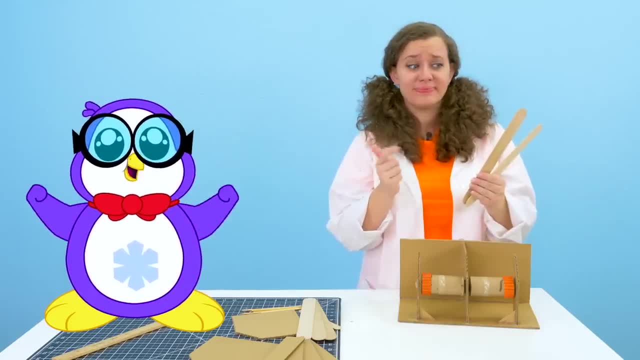 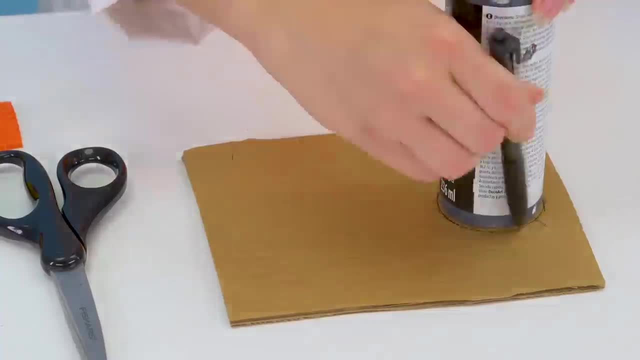 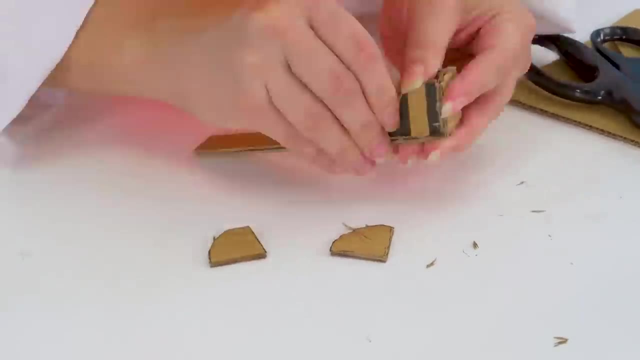 Boring. I think we need to add some color. Yeah, color, pow, Whoa, magic pink. now we're gonna make the part that spins the reel. all we need is a circle Cut into four pieces, and then we're gonna make it 3d. 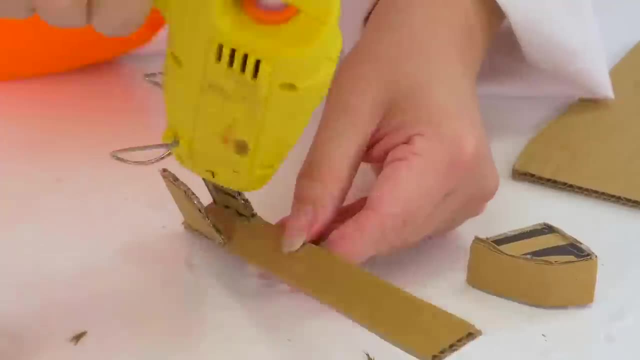 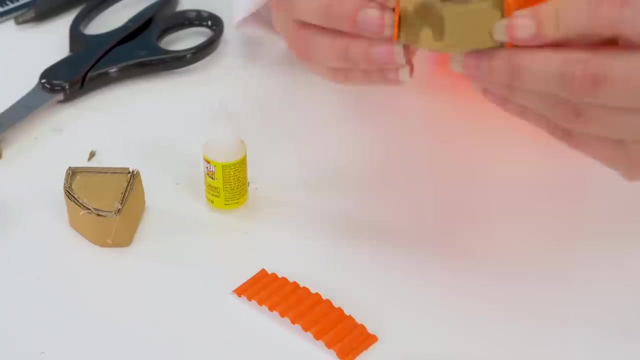 Kind of like a piece of pop Hi. Once we have that all hot glued and dried, We are gonna put the same border paper that we put on our reels. Once we get that glued into place, we're gonna stiffen it with super glue and it should look something like: 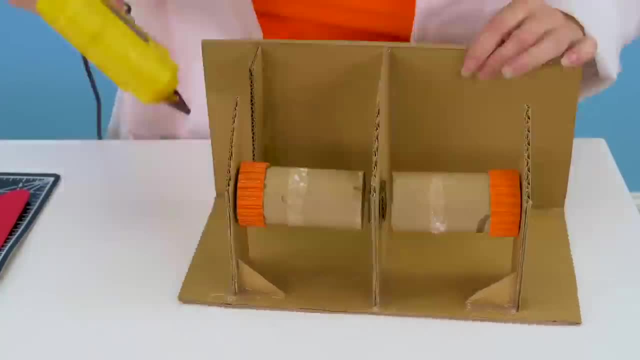 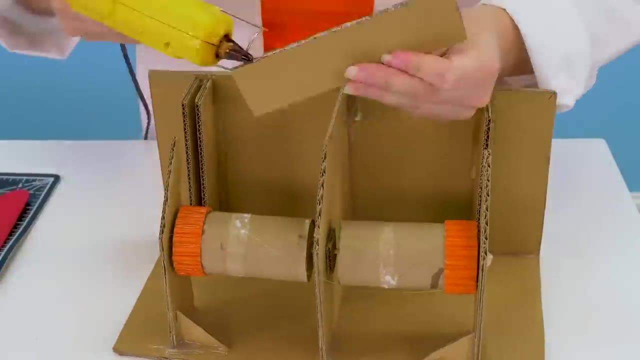 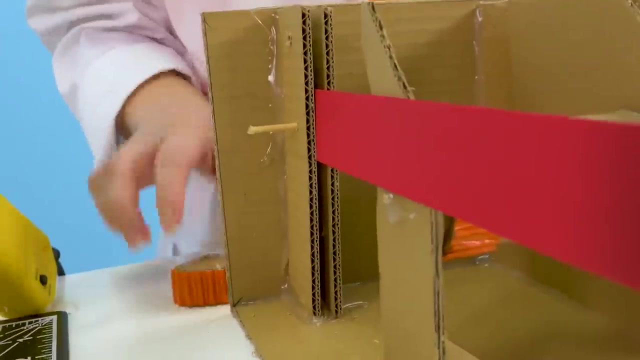 This Whoo, this looks complicated, Whoa, and that's why you have an adult Peck. Oh, All right, Peck. So we got our Levers in place. we use just little sticks to hold them in place. now is gonna be the tricky part. 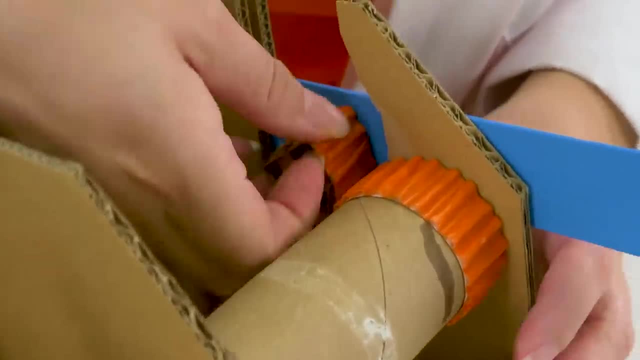 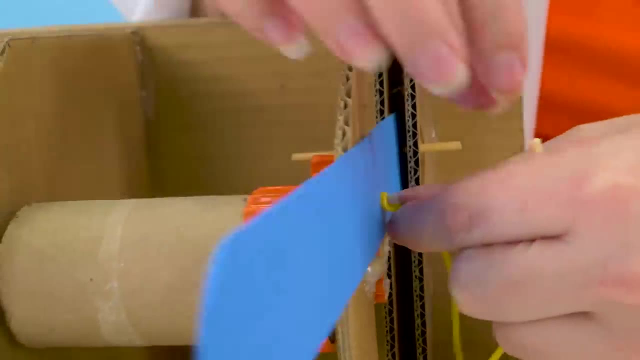 We're gonna have to attach these little tiny gears to the lever. So when you pick the lever up, it spins the reel like that. Now, this rubber band has a very important job and our machine wouldn't work without it. It puts a lot of tension on the lever when you pull it down. 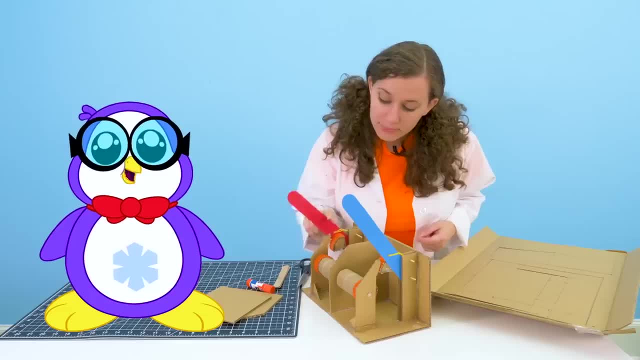 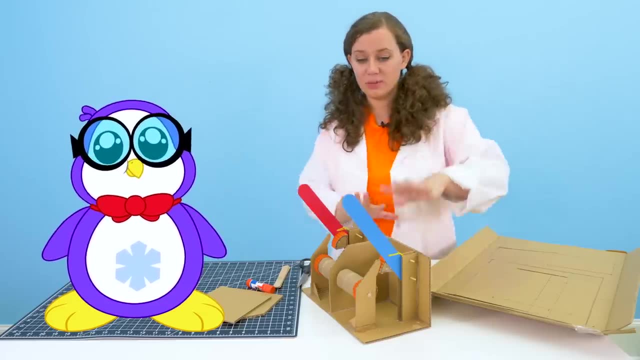 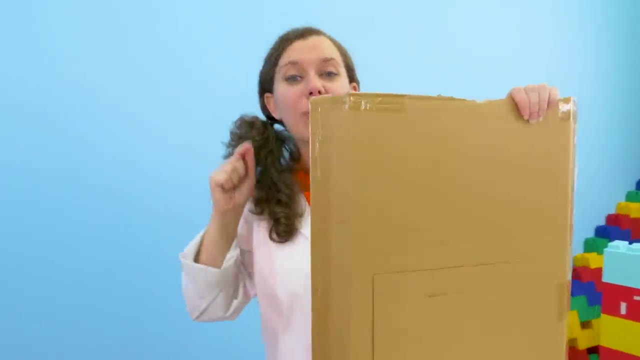 So when you let it go, it spins the reel. the levers are in place and they're working. Yay, What's next Bree? Oh well, all we have left to do is just build the cover Conveniently. I have it all drawn out here, So we just gotta pop it out and here we go. 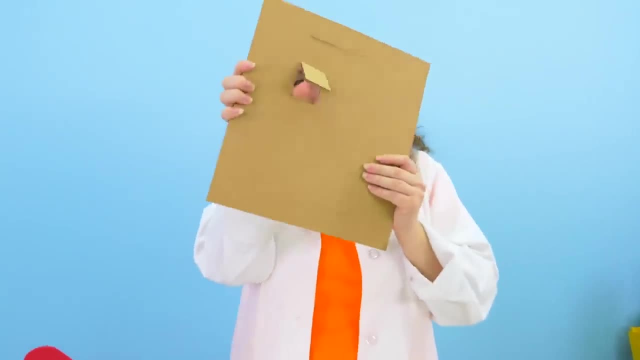 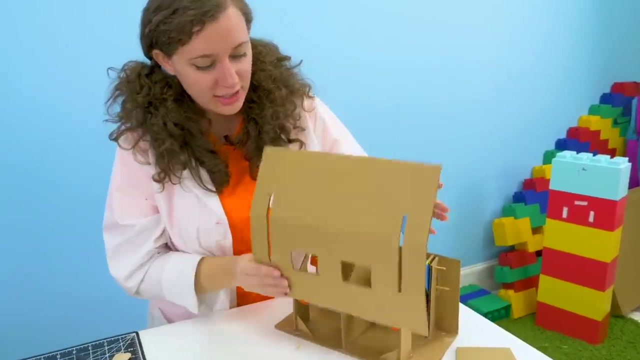 Now, this one has a lot of holes in it, so we gotta punch them out. There you go. So now that we have our cover put on, we can just put this whole thing together. Wait a second. before We can put the cover on, we have to turn it around. 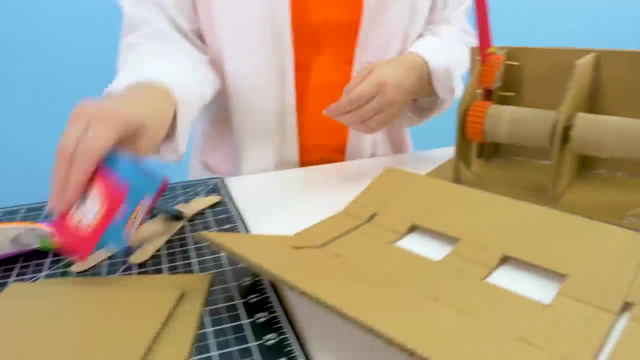 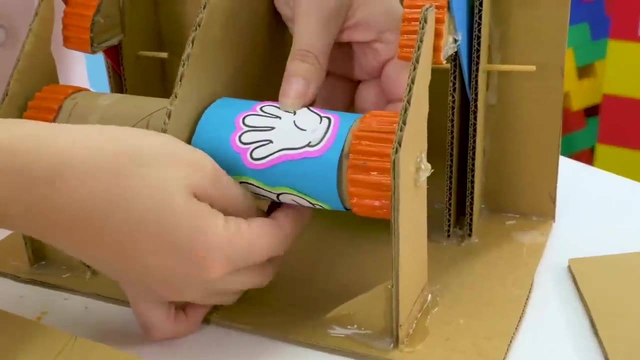 turn this into paper rock scissors. That's where these guys come in handy. We've got rock, paper and scissors, So we're just gonna glue them on like this. The most important part about this step is to make sure that your hands are facing each other. 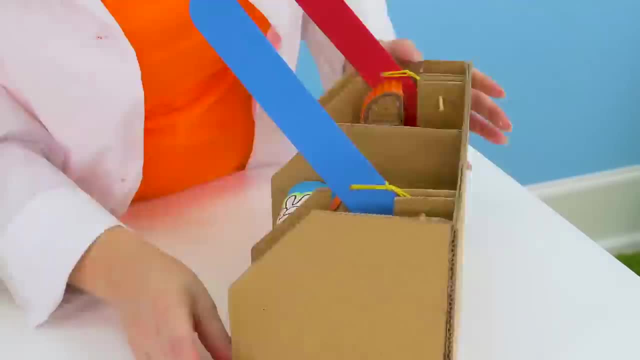 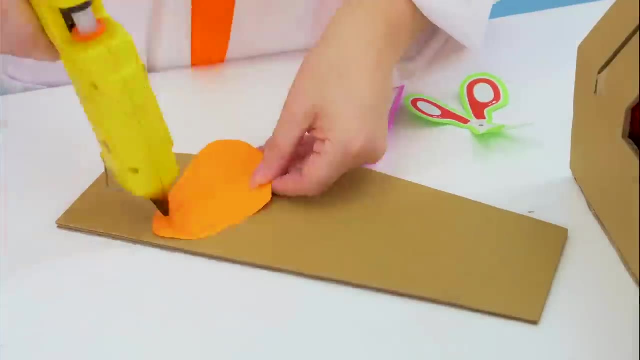 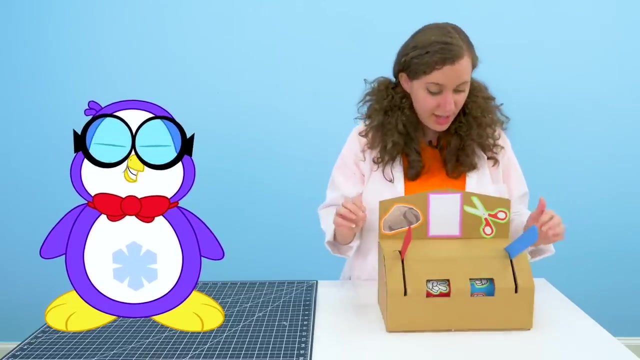 Otherwise, who are you playing? Now we're just gonna glue the outside pieces of our machine and the front cover. Wow, it's really coming together. And we can not forget rock paper and scissors. The rock paper scissors machine is complete. 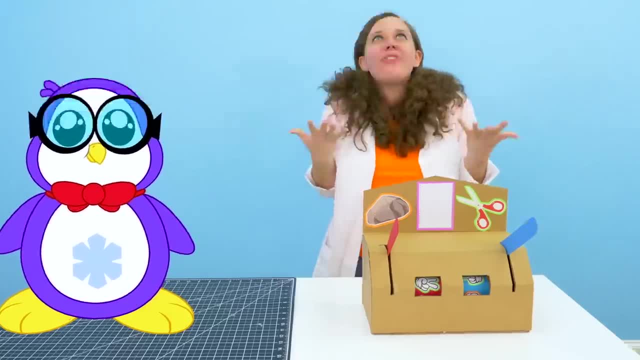 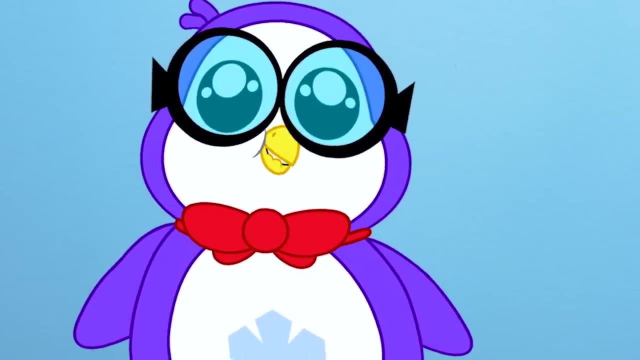 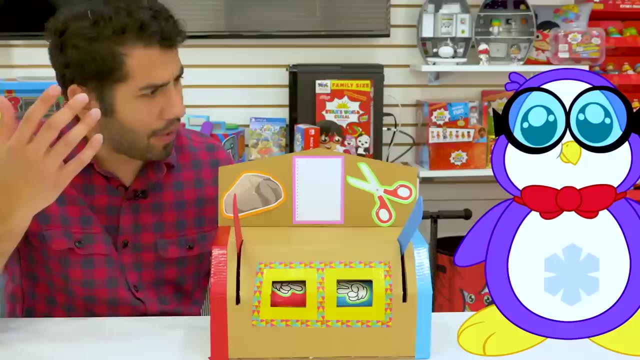 Now let's decorate Some decorations. My favorite part, There it is. We have red versus blue, Boom, Woo hoo. Hey, before we give it to Ryan, I should test it out again. Okay, well, good luck.